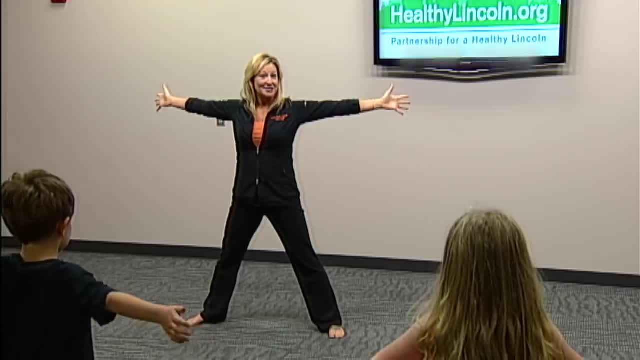 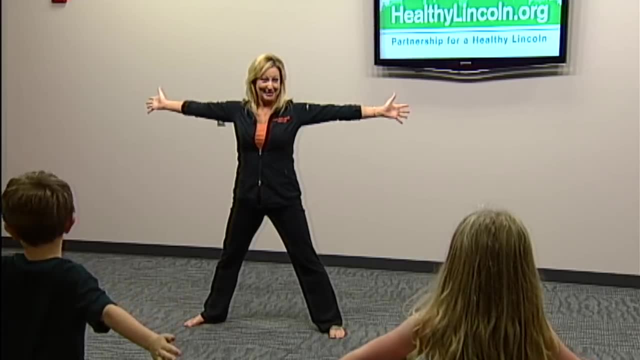 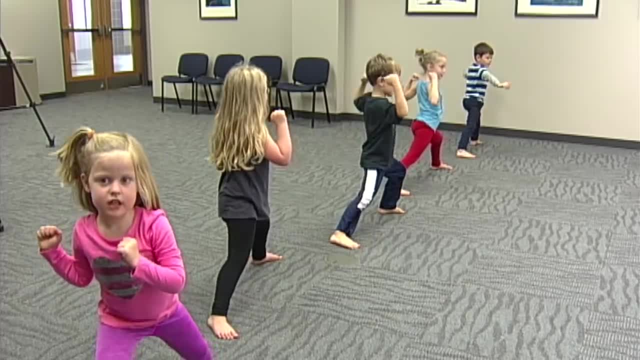 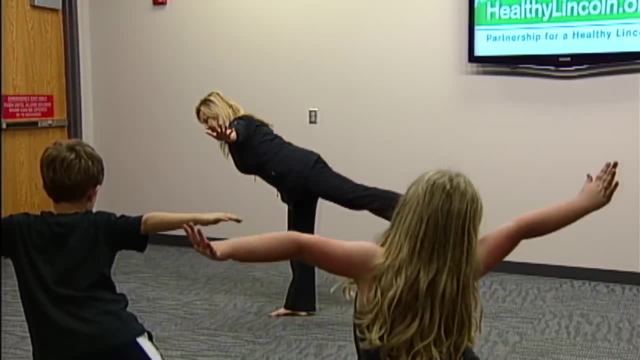 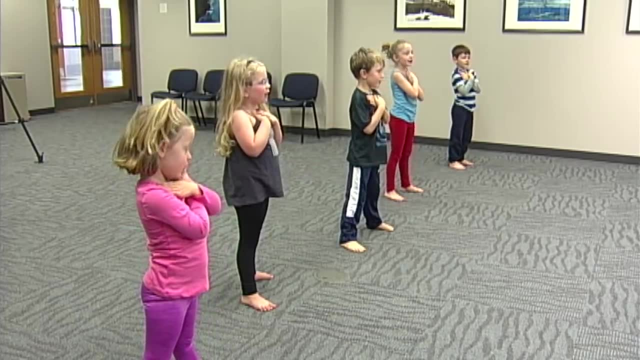 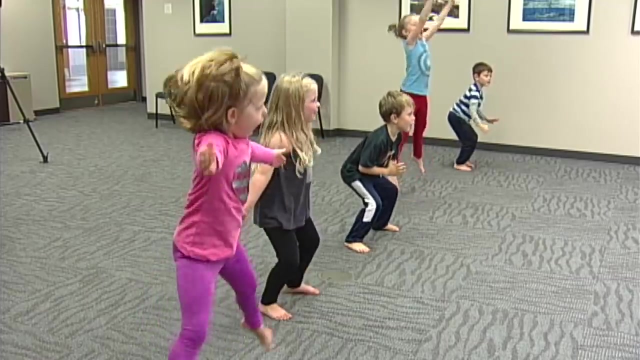 see if we can balance, Coming up and say I am balanced, I am balanced, Good job. Step together, Hands come to our heart, Say I am kind, I am kind, Good job. And then hands come together and we jump out in volcano and we say I am me, I am me Nice, Let's do it. 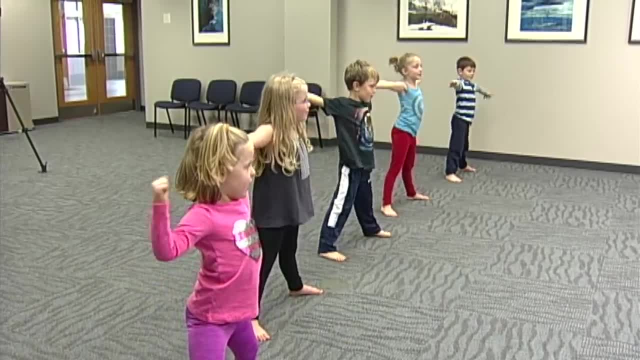 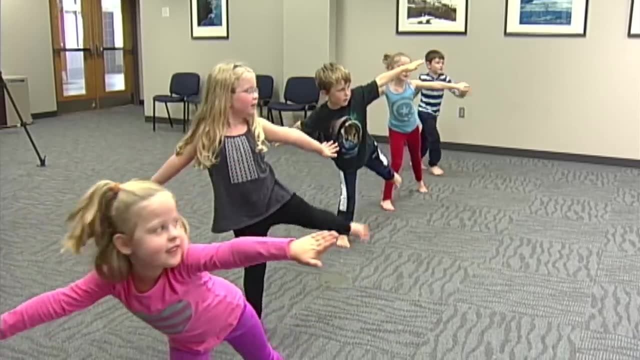 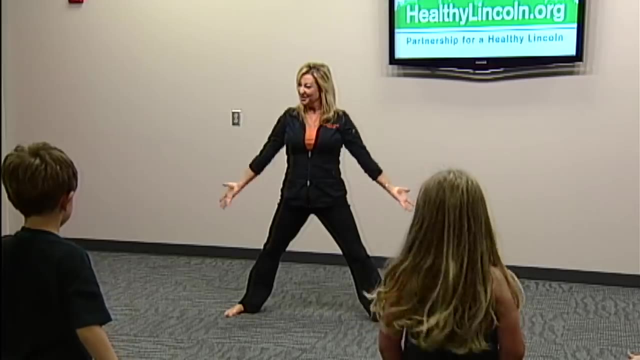 one more time. Okay, ready, I am bright, I am bright, Let's go this way. Go ahead and let's go this way. I am brave, I am balanced, I am kind, I am me. good job, and there's only one of you, so it's really important to do healthy things and take 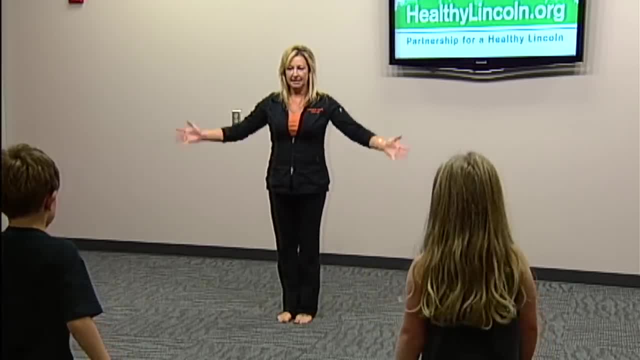 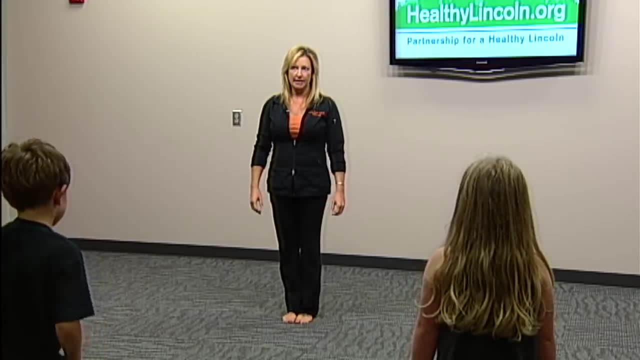 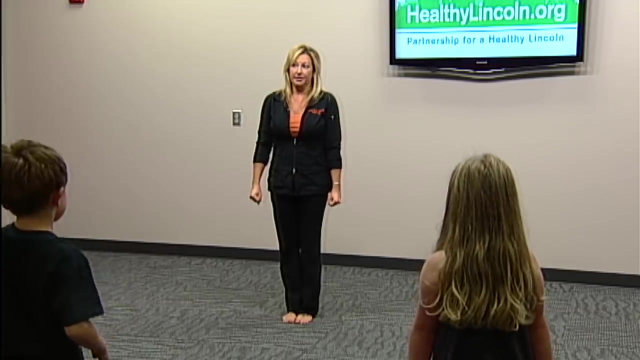 care of yourself, right? so let's bring our feet together. this is called Tadasana, our mountain pose, so we're tall and strong in our mountain pose. so what happens when we get frustrated? what's our body do? what's our breath do, right? are we gonna make a good choice when we're holding our breath and our bodies? 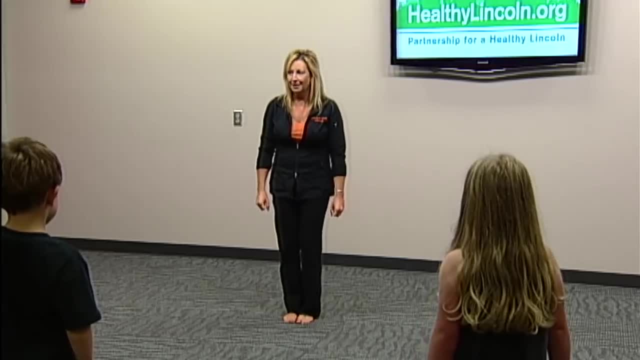 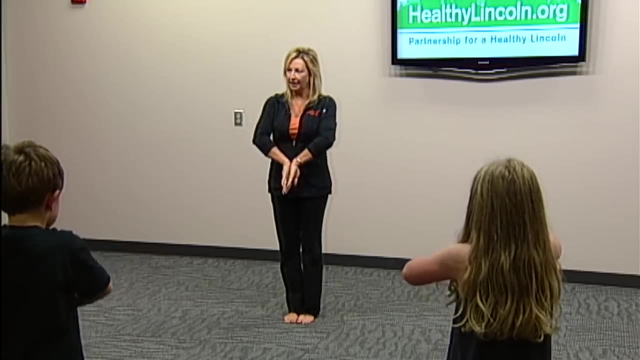 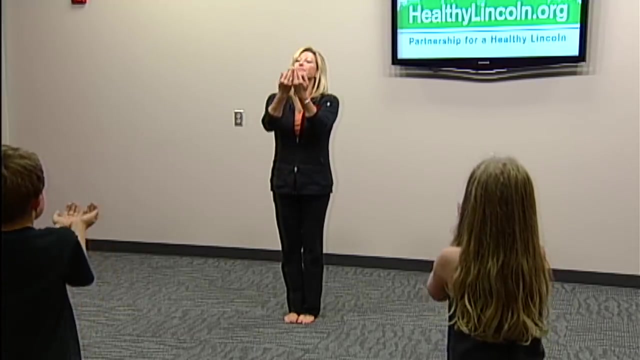 like this, right? so the first thing we need to do is make sure we're breathing. so take your hands out in front, open your hands towards your heart. backs of your hands come together and dive them down. good, bring them back up and out, so we're gonna breathe. with this ready, breathe in, breathe out. 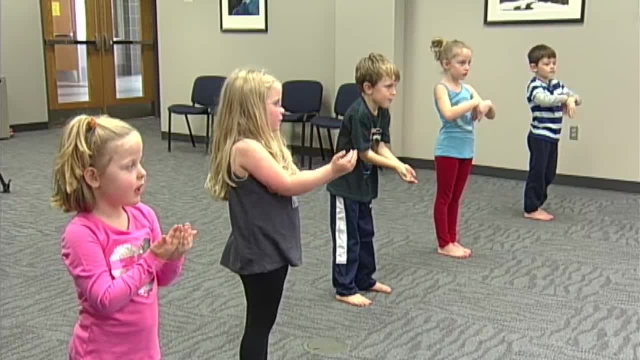 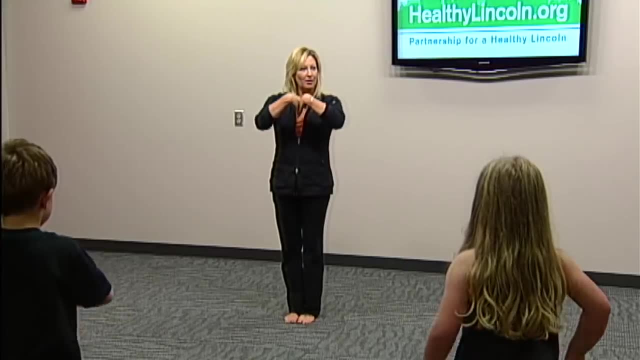 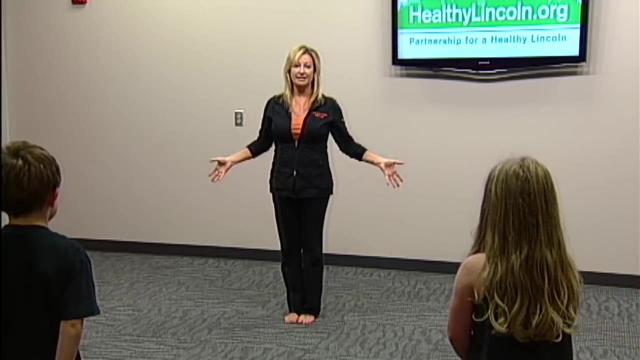 breathe in and breathe out good. so we're bringing in what we need towards our heart. right, letting go of the things we don't need and filling up our heart so that we can give right, all right. so the other thing we can do when we get angry or upset is shake some of that stuff off. so we're gonna do happy. 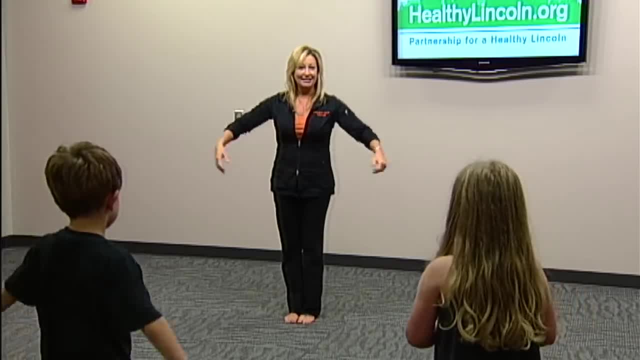 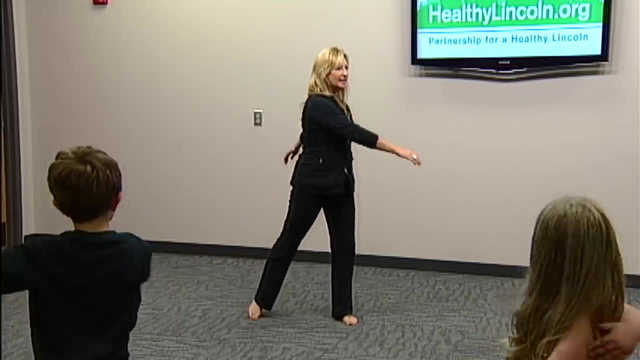 elephant, so make sure you have enough room so you don't hit each other, and these are gonna be our giant elephant ears, all right, and we're just gonna swing our arms back and forth. anything that's frustrated you or made you upset today, let go of it here, shake. 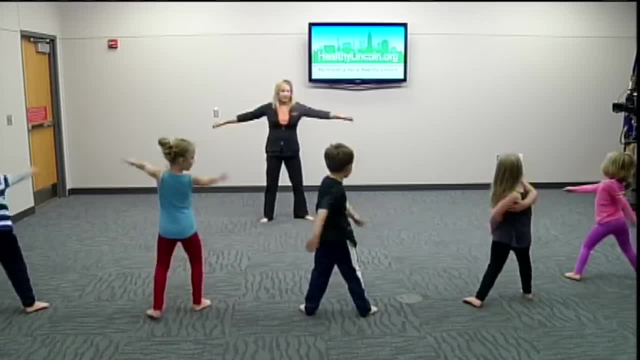 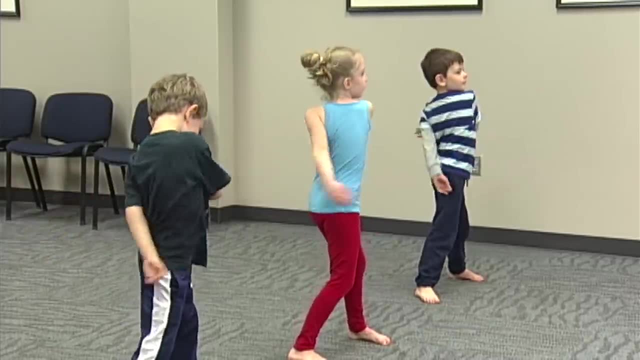 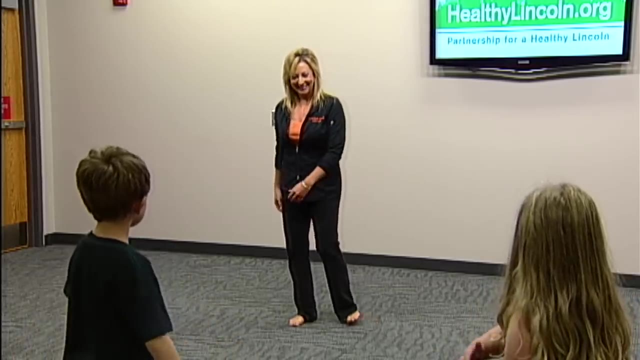 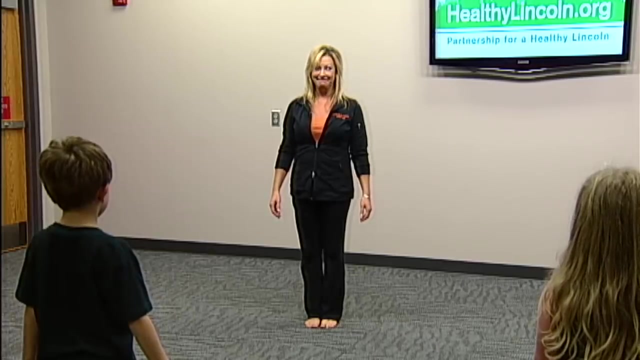 it off like it's moving out your fingers back and forth. all right, start to slow down our elephants getting tired. good, step your feet together and now close your eyes and notice how your hands feel what's going on in your fingers and your arms. good, open your eyes, did they feel tingly and your arms feel like they wanted to float. 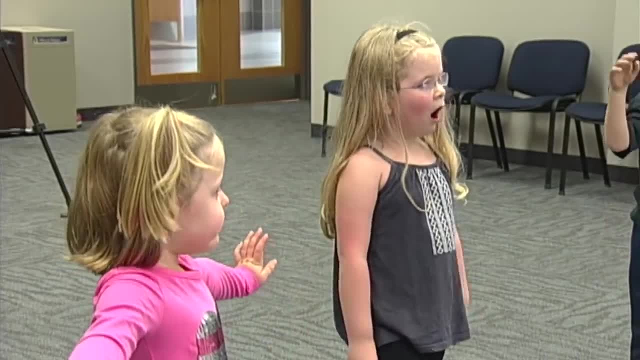 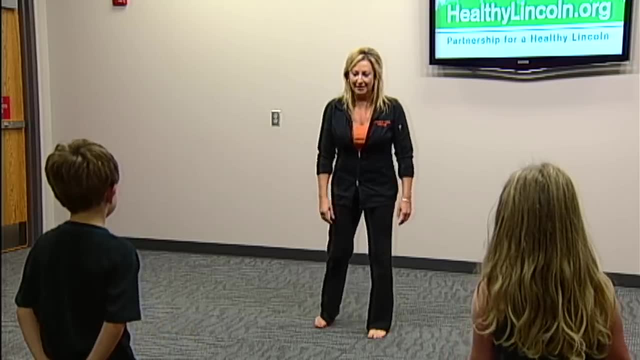 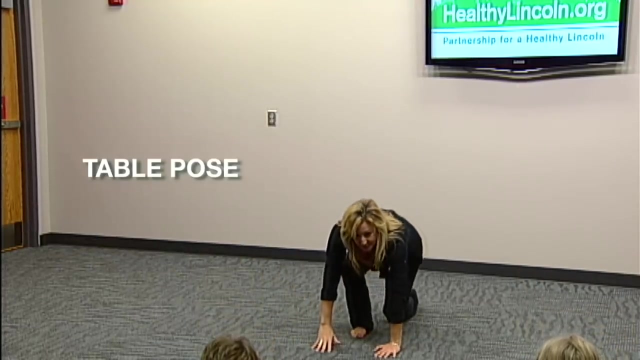 up, right, yeah, so we want to listen to what our body is telling us. so pay attention when you're hungry, when you're tired, those kinds of things, so that we take care of ourselves. all right, so bring your arms up and bring them down. are we ready to come back to table pose? so here's our table pose. so cat and cow. 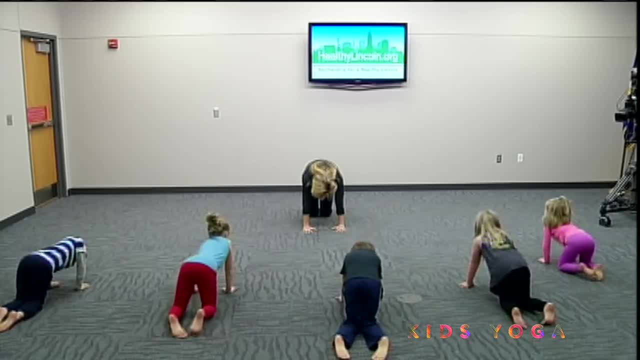 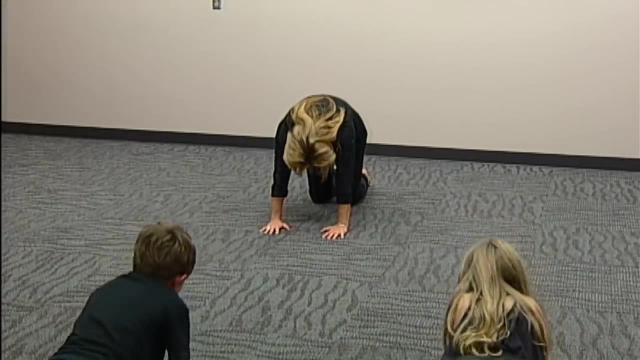 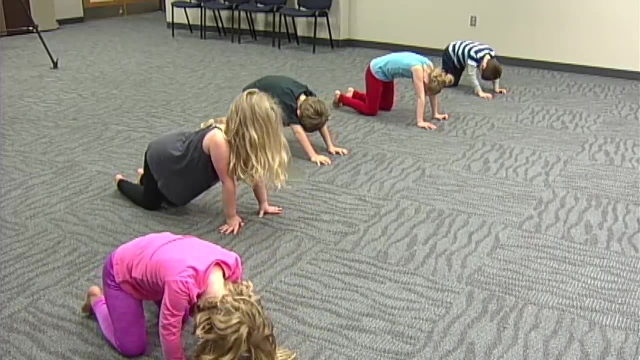 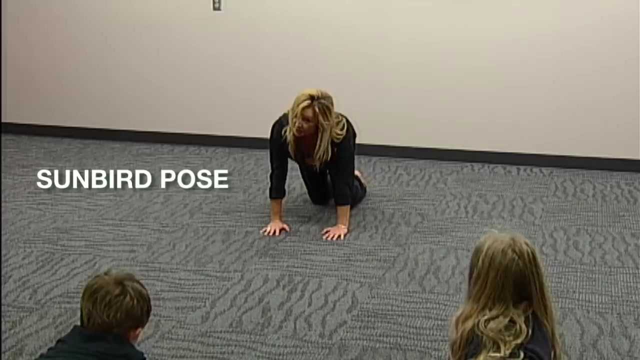 so we arch our back like a cat and then cow pose. come forward like your belly full, belly's full of milk. moo and cow pose, good ready. meow and cat, and then moo and cow- good. one more time: cat and cow, good job, all right. so sunbird. so with sunbird we're doing opposites, so same side is. 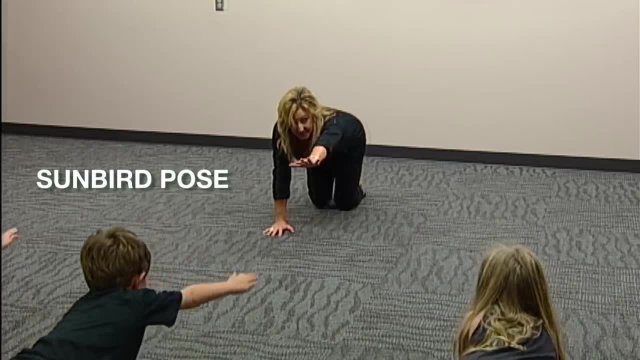 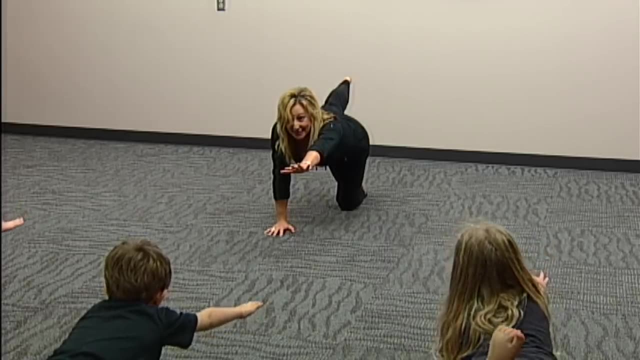 really hard to balance, so we're gonna take one hand out and then I'm gonna take my opposite leg out. there you go, good job, Henry, and breathe good. and this one you can even do with the friends, so you can like hold each other's hands and see if you can help each other to balance better. good, okay. 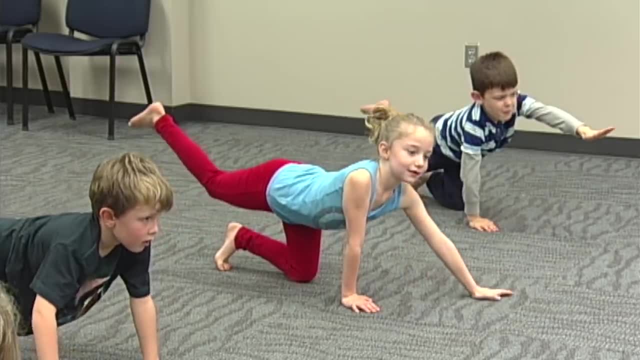 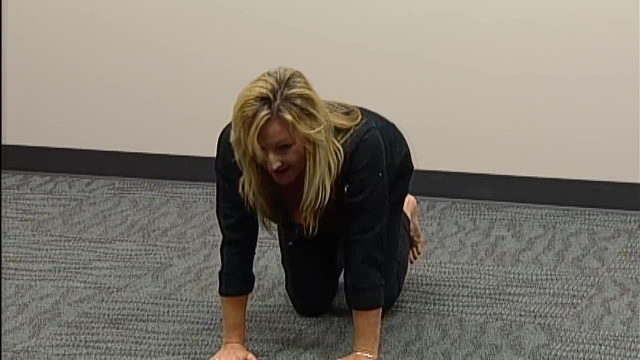 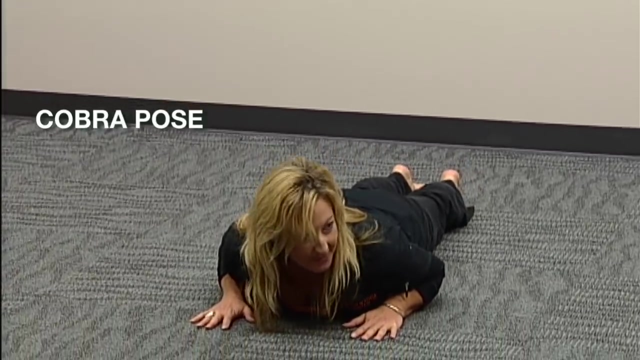 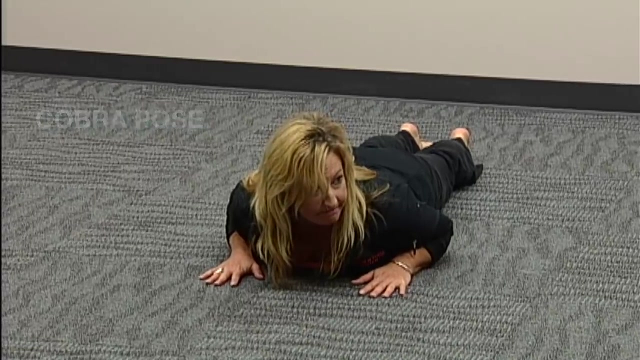 other side reaching out. good job breathing, and all right, let's come down on to our tummies. so we're gonna do Cobra pose and Cobras the type of snake right, yep, yep, do Cobra's have? or snakes in general, have arms? no, all right. so we 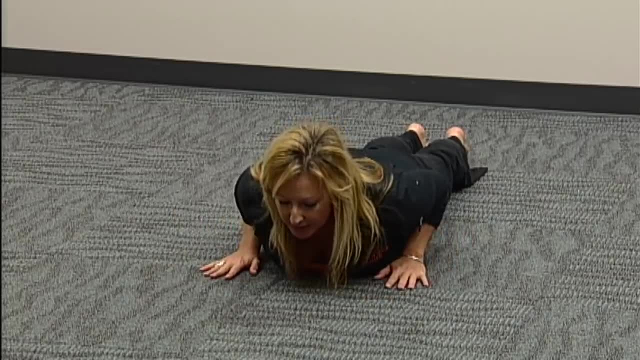 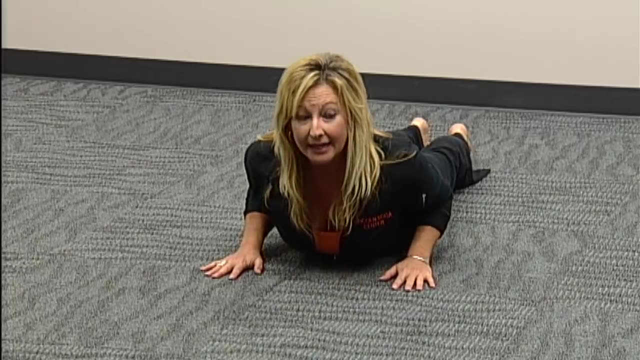 want to keep our big snake tail down, so our legs stay down and our elbows hug in towards our bodies, cuz we're snake and we don't have arms, all right. so when you breathe in, lift yourself up with your muscles in your back. and now, when you 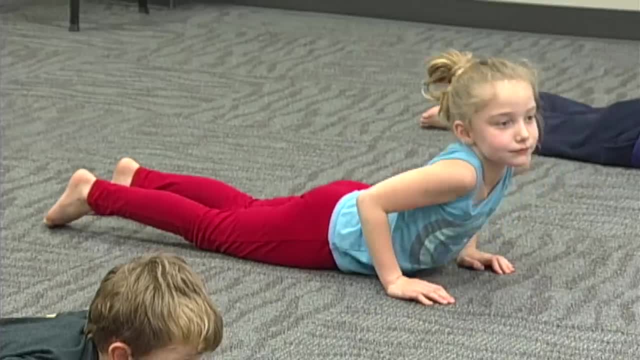 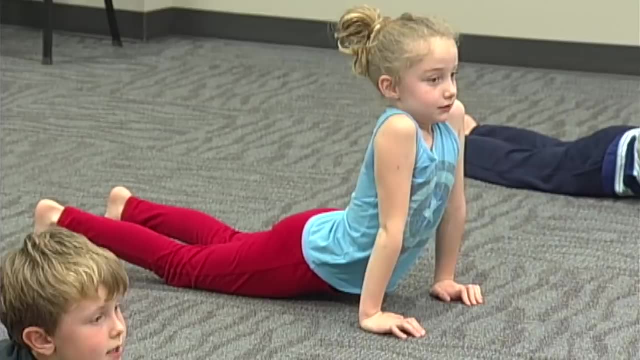 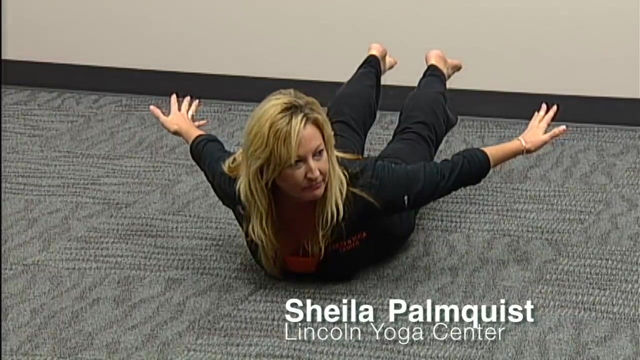 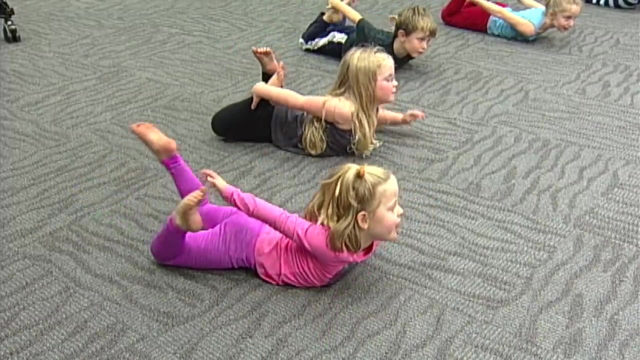 come down like a snake. all right, let's do it again. breathe in, and now good, one more time, big King, Cobra, as high as you can. and then nice job, all right, arms, come out and lift up superwoman, man, girl, boy just playing, super right, all right, reach back and grab your ankles. oh, bow, pose that. 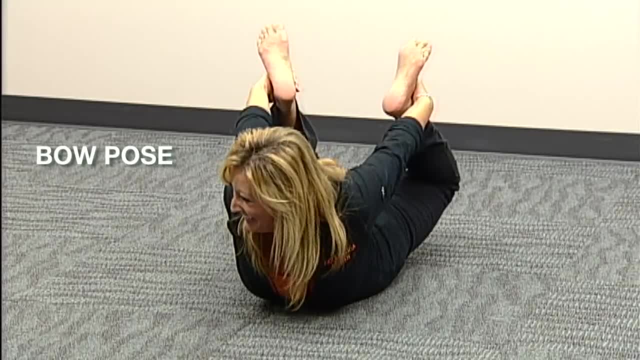 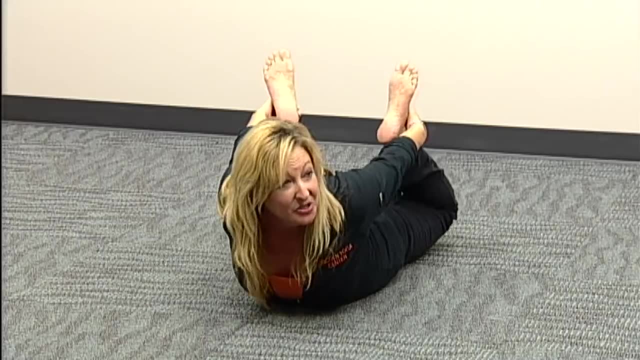 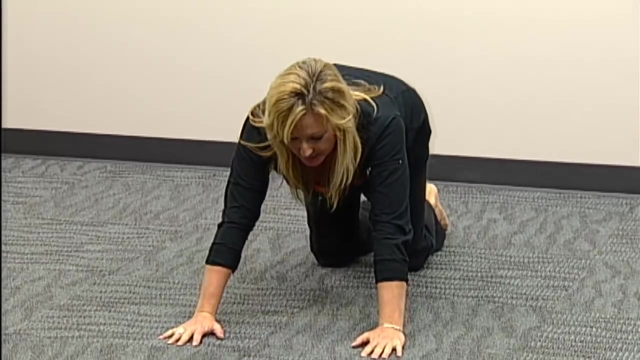 one's kind of hard, huh, so this. so yoga should never hurt. so if you reach back and you go, oh, this hurts my body, then don't do it, okay. so again, we want to take care of our bodies. All right, let's come back to our table pose. 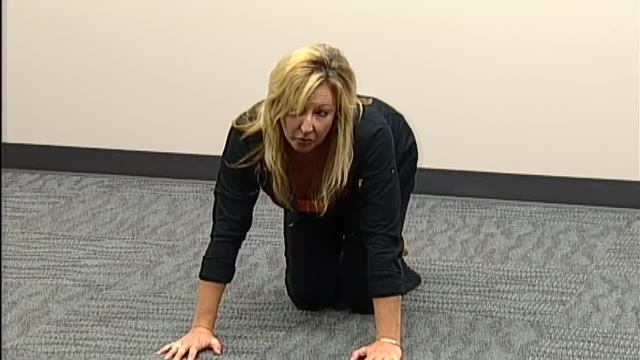 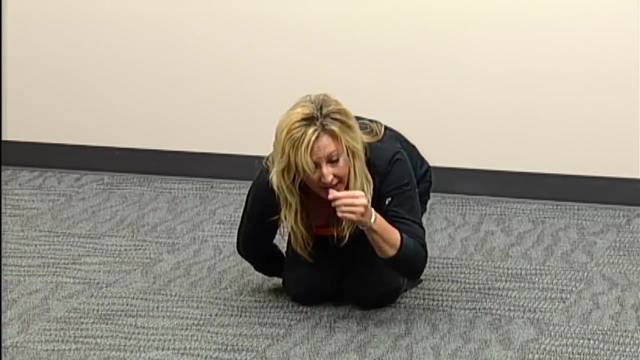 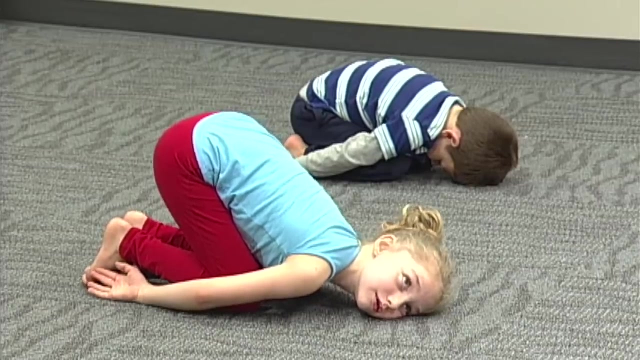 We're going to sit back into child's pose, or sometimes we call it rock. So if you come down like this and rest your head and just breathe here- So imagining if you were a rock, that means all of the rain, the wind, everything would just roll right off of you, right? 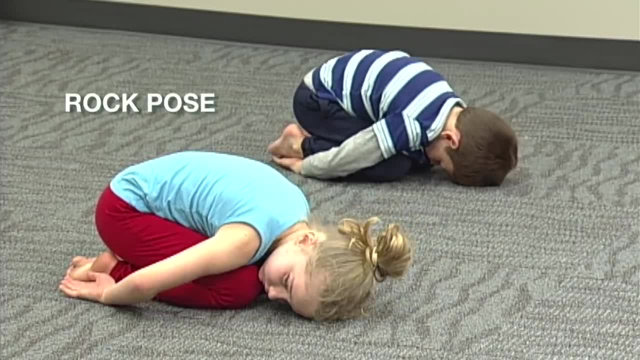 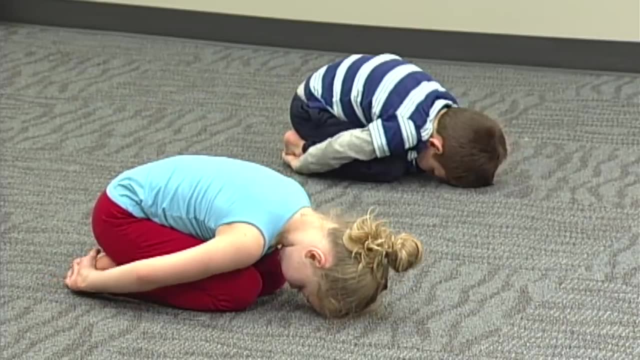 So sometimes when you feel like you need to take a break or take five, you want to come down into your rock pose for a little while. Well, everybody needs time to rest. Good, slowly coming up. Good, all right hands come out in front. 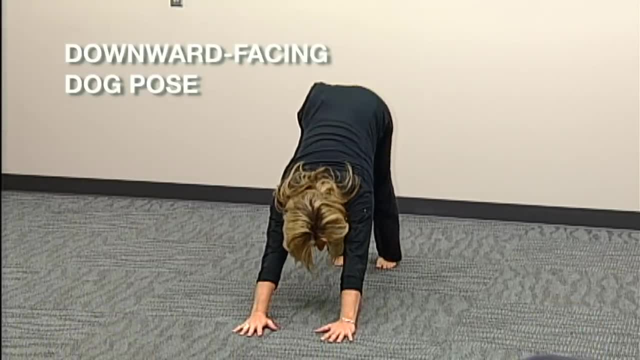 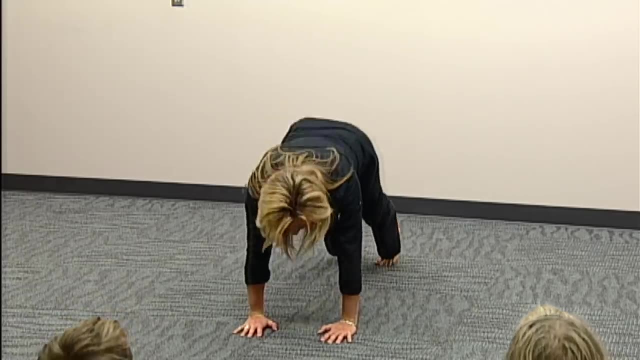 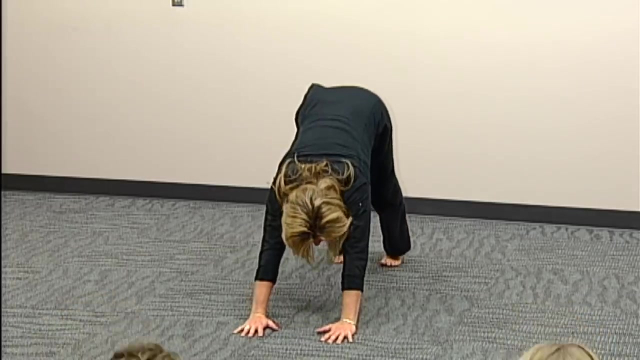 Tuck your toes down dog, Stretch into your down dog And now come into your up dog, stretching like a dog does Good. down dog And up dog, Good job. let's do it one more time: Down dog. 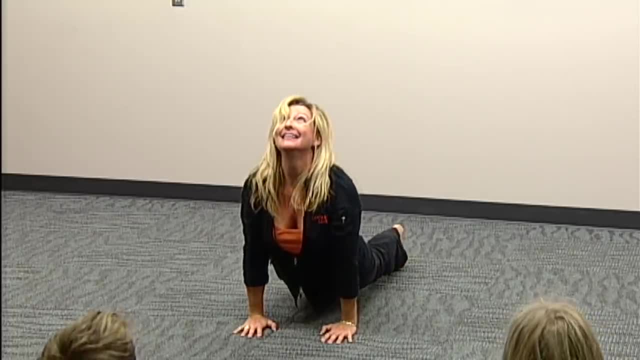 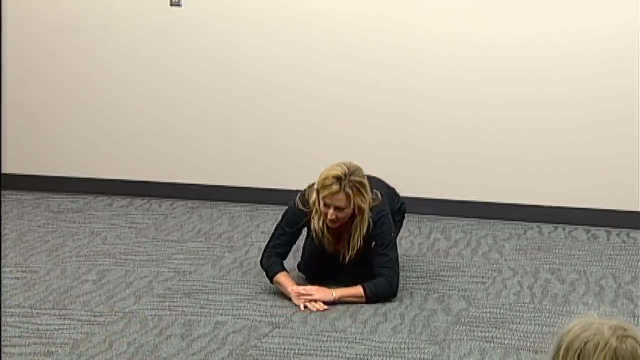 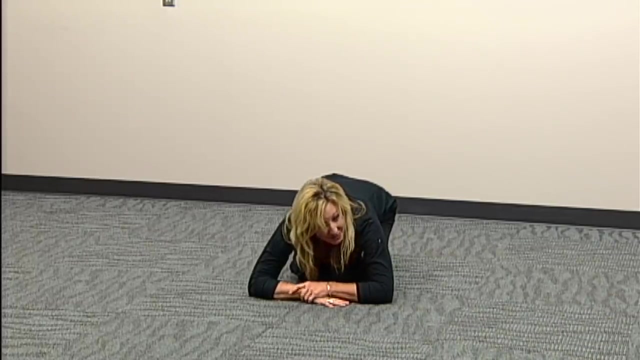 And up dog. Good, okay, put your knees down. And now, this time, instead of being a rock, we're going to be a seed. So come down. And what do seeds need to grow? Water And what else. 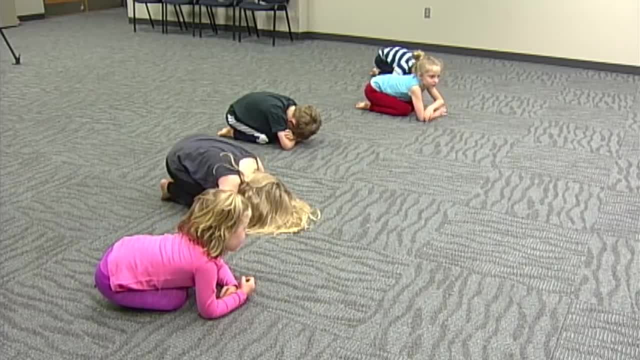 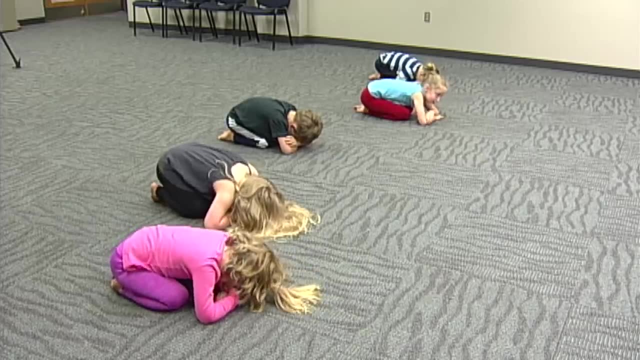 Food. And what is our food? Sunlight, Sunlight and water. So let's wiggle our seed into the dirt. Wiggle, wiggle, wiggle, All right. so imagine we're starting to grow, So start to pop your seed out of the dirt. 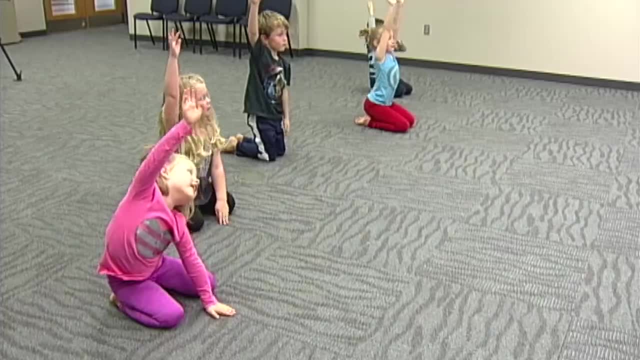 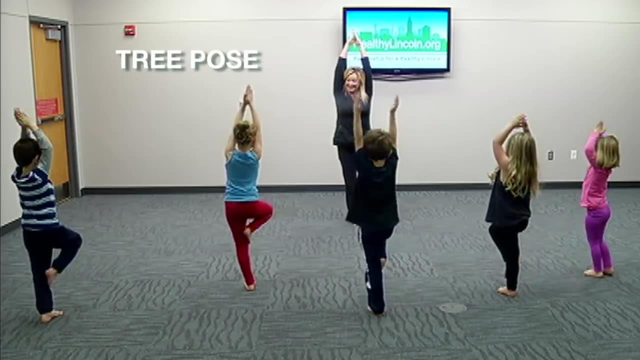 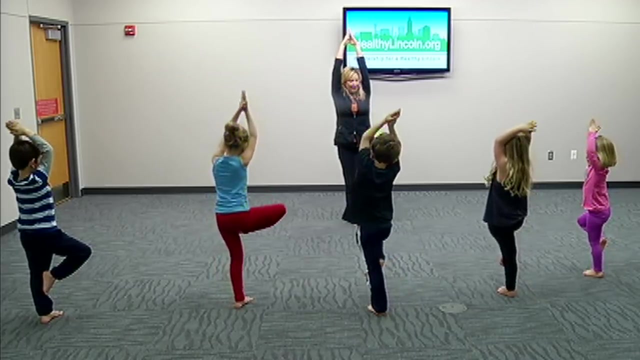 One arm up, Good, and then the other branch Coming up. You ready, Other branch, And we're in tree pose. Nice job, Yeah, Awesome. I'm glad you're practicing yoga. It's fun, All right. so what are the leaves doing off of the trees right now? 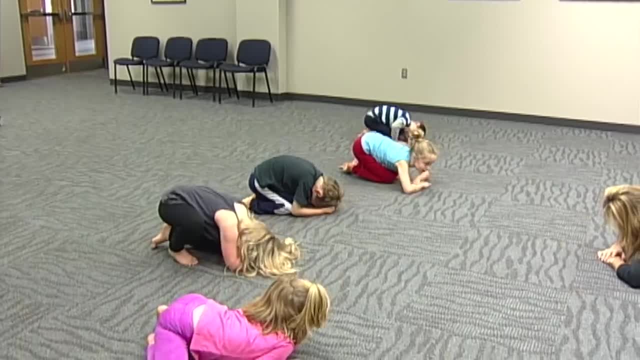 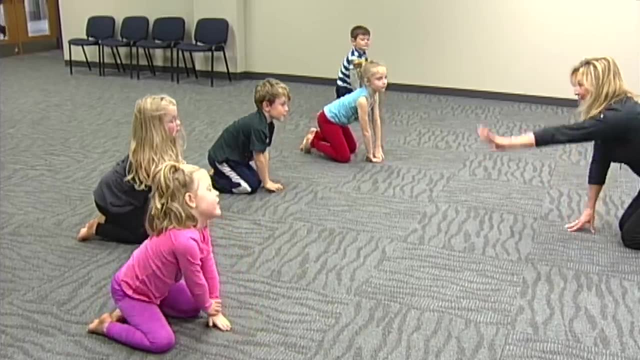 Falling, Fall, Let's come down. Okay, Let's wiggle into the dirt And let's try to do it again and lift our other leg. So here we go, We're starting to grow, Coming up, Popping one branch out. 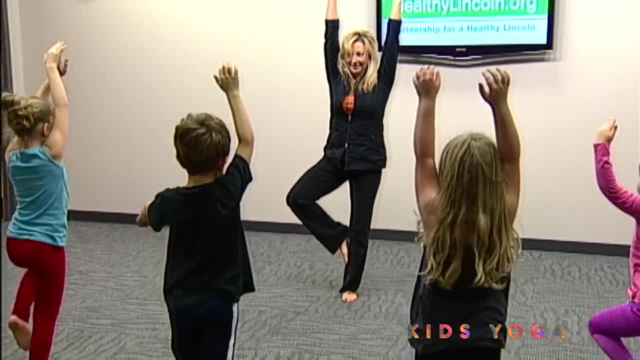 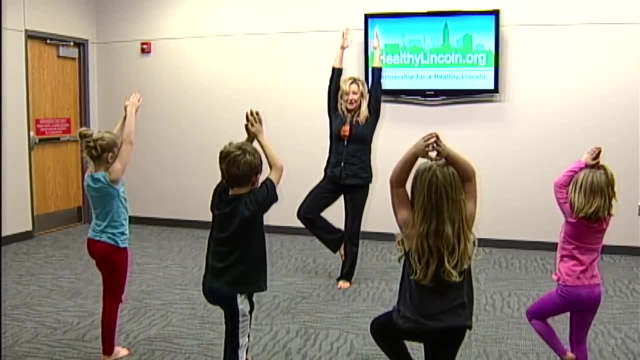 And another. See if you can remember which leg to lift, Lift Tree pose. Sometimes it's windy in our tree, That's okay. If we fall, we get back up again, right, All right, What did I just say? 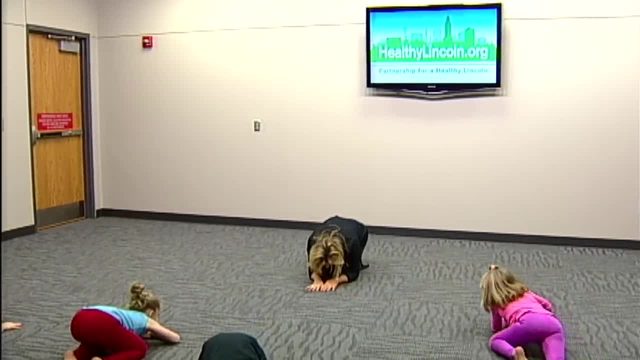 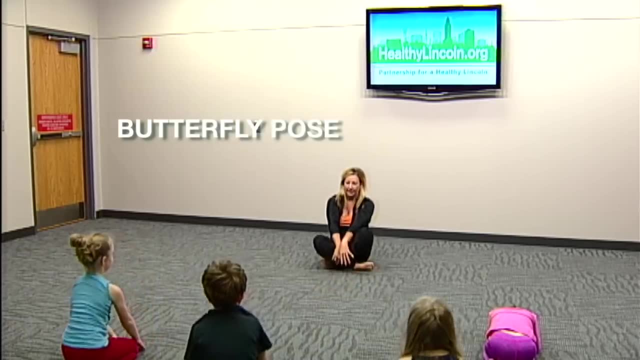 Fall. Let's come back down. Good, All right. So from here let's go ahead and look at our tree pose. All right, All right, All right. So from here let's go ahead and come into our butterfly pose. 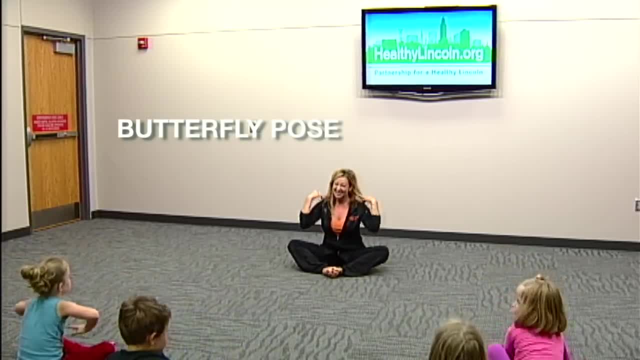 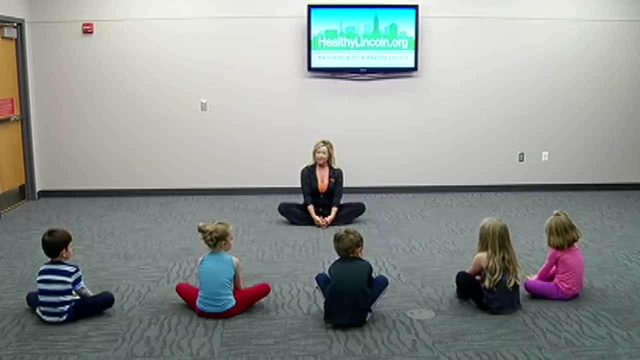 I can do that dance. Yeah, I used to do this in gymnastics a lot, So, butterfly, I can have a butterfly dance too. Good, So butterfly wings. And we want to be gentle. Remember, yoga should never hurt, All right. 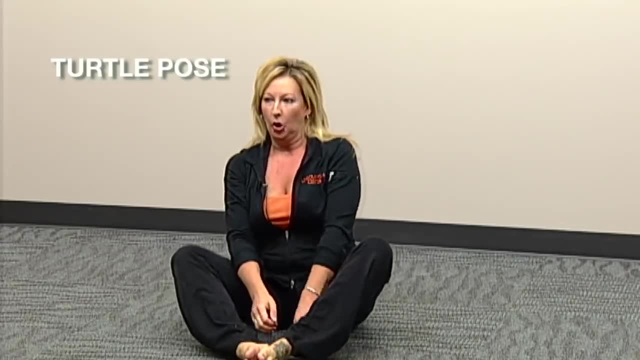 So now we're going to do turtle, Bring your arms underneath, Good- And we're going to round our head and put our head in our turtle shell And then start to think and look out of your turtle shell Like, ooh, what's out there? 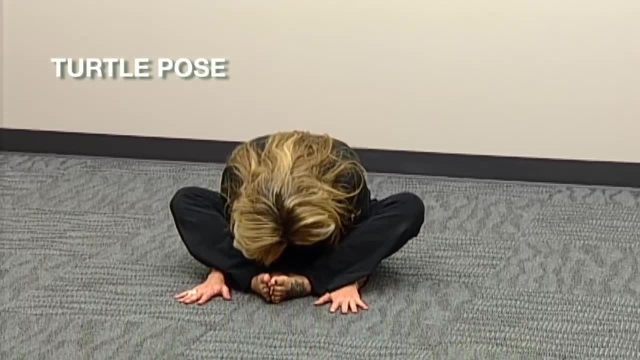 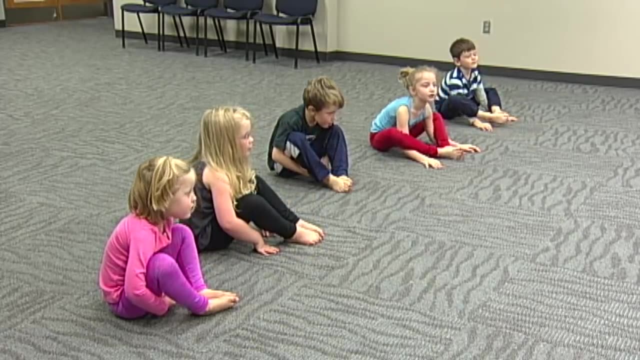 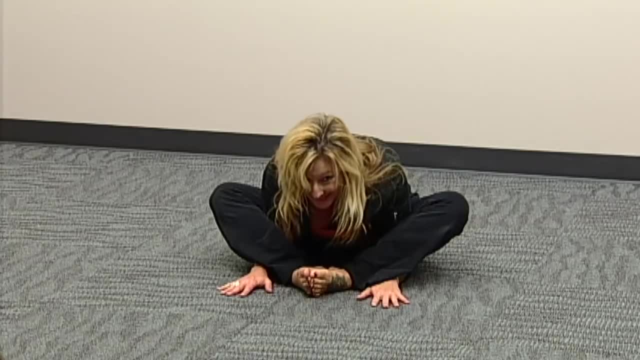 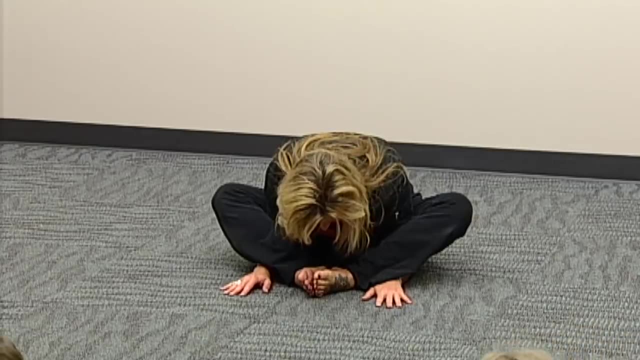 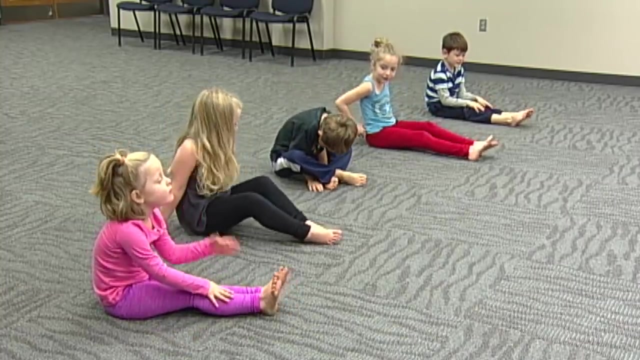 scared and they go back in their shell. bring your head back down, good, and then start to lift up so you feel the stretch across your shoulders when you lift up, yeah, and come back down, good, take your arms out, all right. it is, yeah, and it feels good for our bodies, all right. so our next pose or exercise that we're. 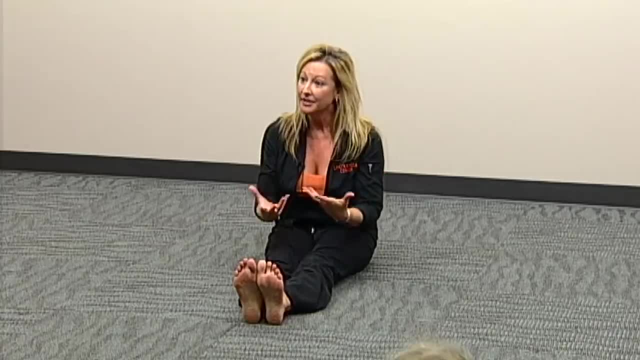 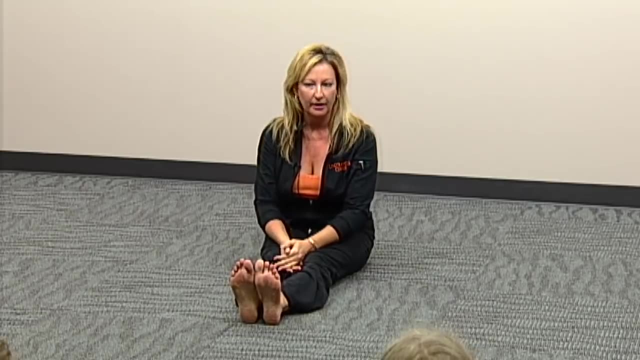 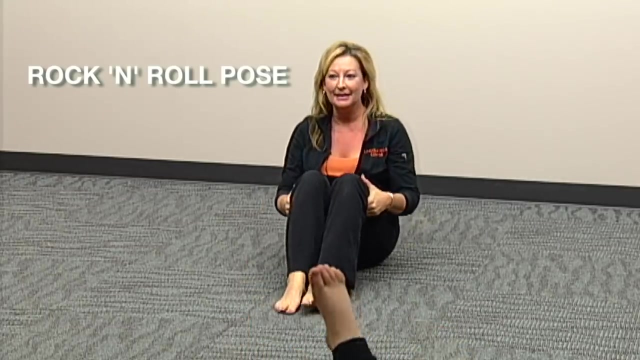 gonna do is called rock and roll, and so this is another thing you can do if you feel like you're frustrated is to just be playful and roll around, because if you start to get silly, you kind of forget why you're upset. so our hands come here. yeah, we're gonna rock back and come up good. rock back and come up good. 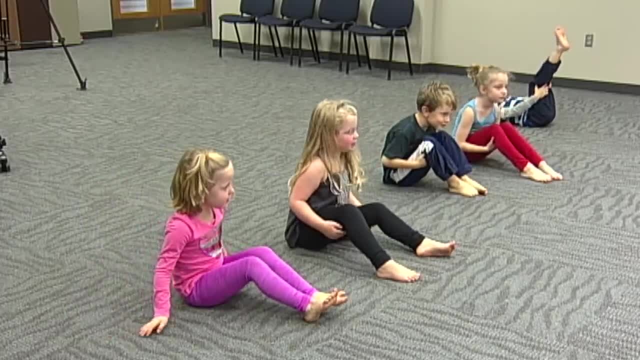 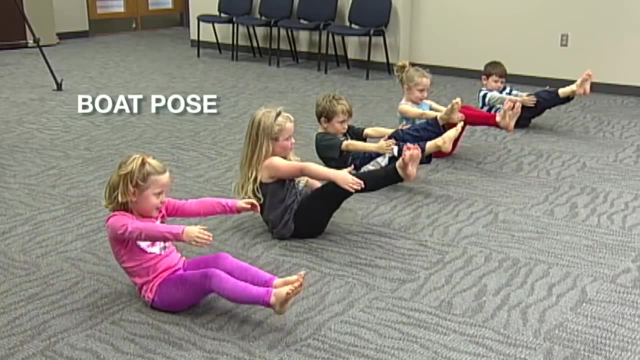 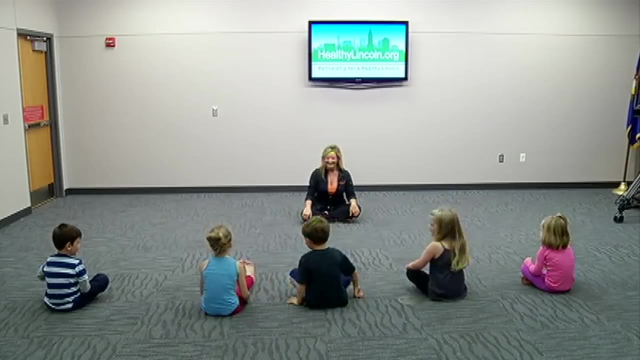 rock back and come up. can we stop in boat? let's rock back and let's come up and stop in boat. oh, that's kind of hard, right? we have to use our tummy muscles. good, all right, that's good, okay. so let's come on to our knees and our 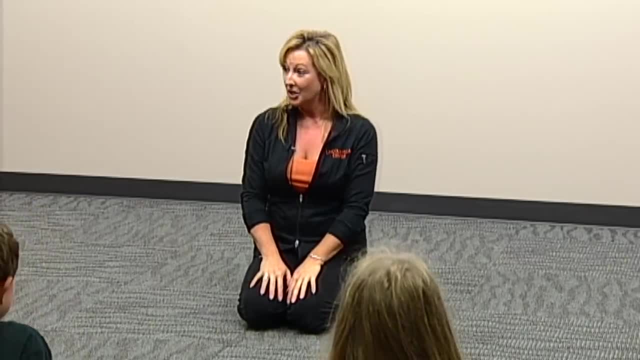 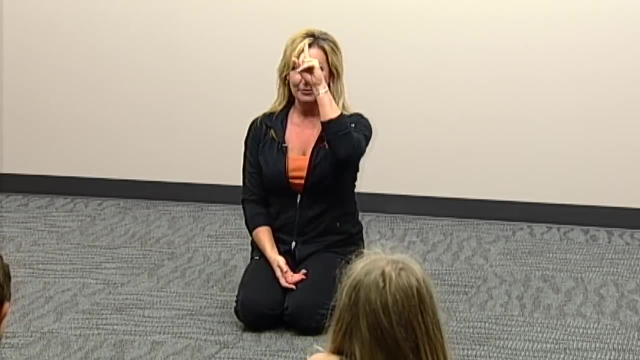 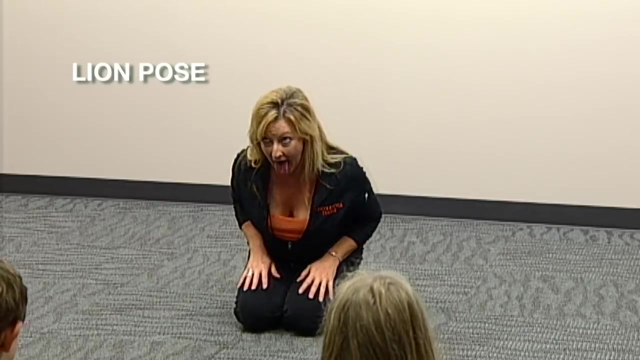 next breathing practice- speaking of being silly- is called lion. so it's fun, isn't it? so it's kind of silly. we stick our tongue out and we look up. all right, these are our giant lion paws. so we're gonna breathe in and then we're gonna go. 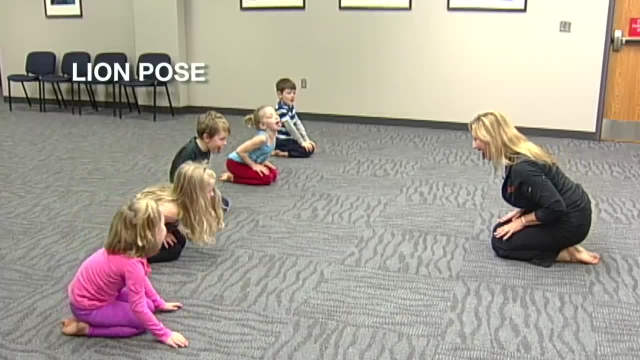 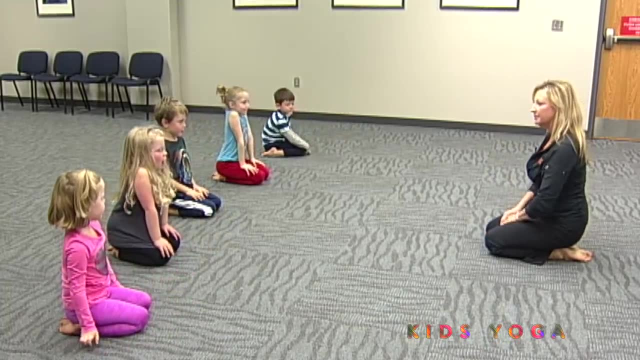 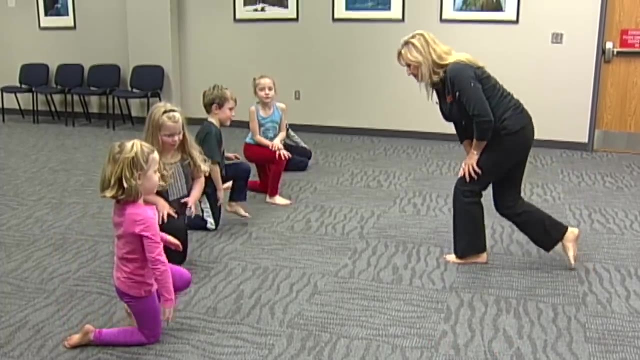 ahead, let's do it again. good, that's fun and that's silly. one more time. good, and it feels good to sometimes growl. right, we need to do that sometimes, as long as we're not growling at someone, all right. so let's stand up and we're gonna do our. 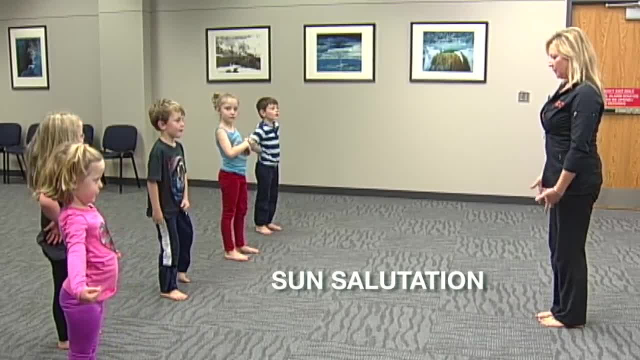 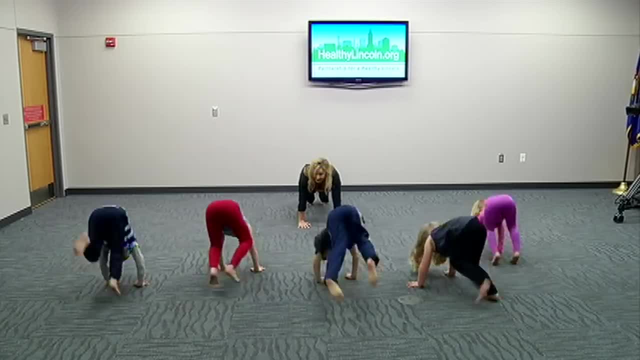 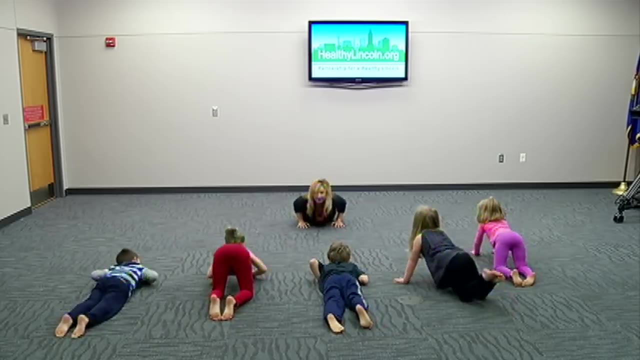 sun salutations. so you might know this one too. bring your arms up and come down, and you can hop or step your feet back, all right, and then we sit back. so remember this one. here's kind of a rock pose, and now we're gonna slide forward. and here's our Cobra breathe in good job. here's our. 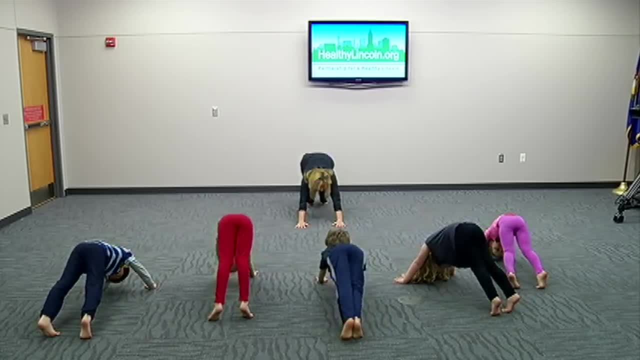 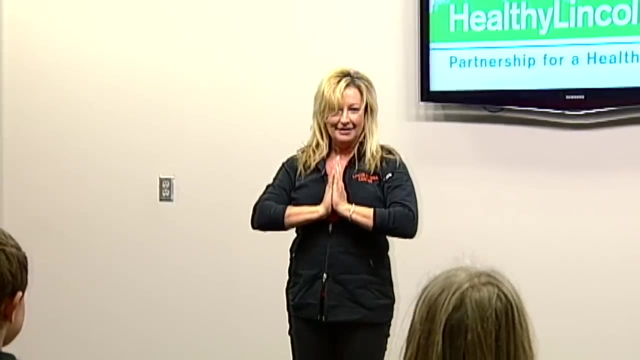 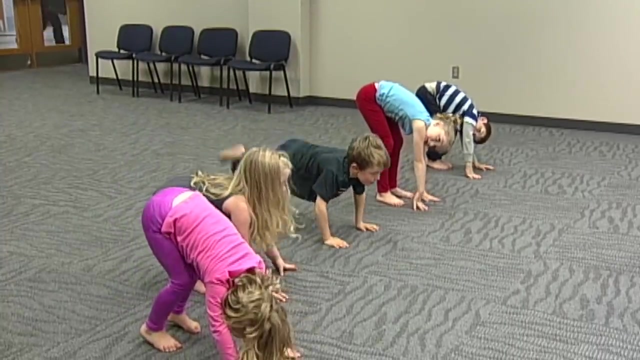 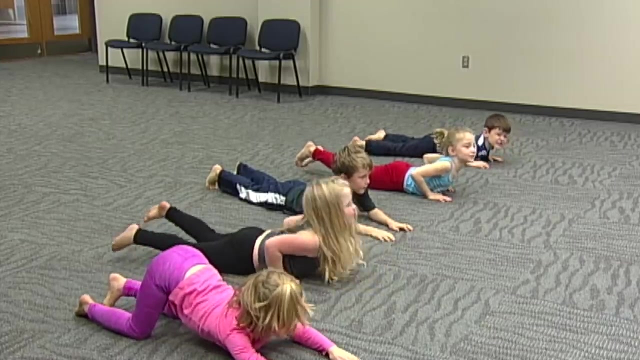 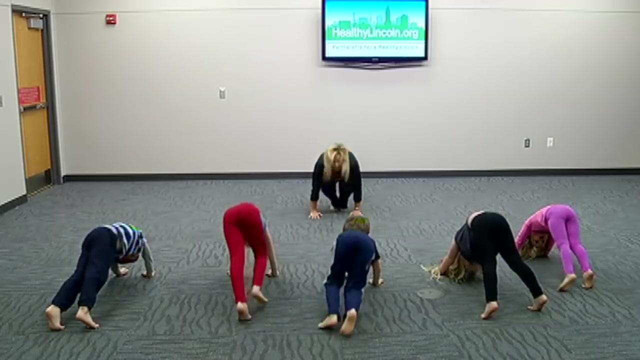 down dog, and you can hop or step your feet up. so there's no competing in yoga. do what feels good for your body today. all right, do we got that? you think we can do it again? okay for you, then, and come up to standing. cut off that awesome. 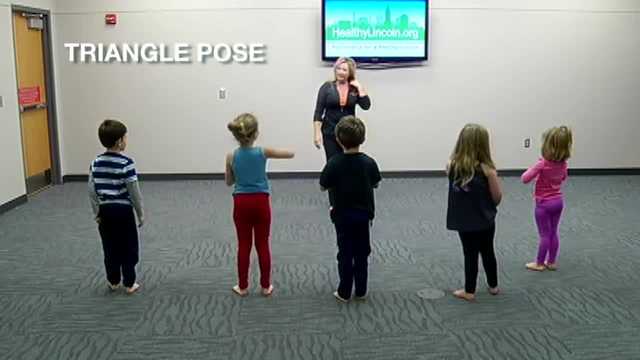 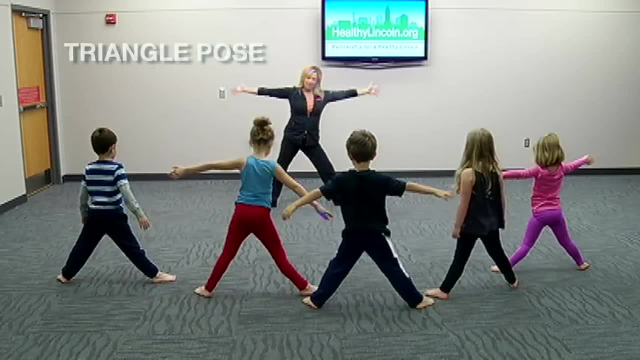 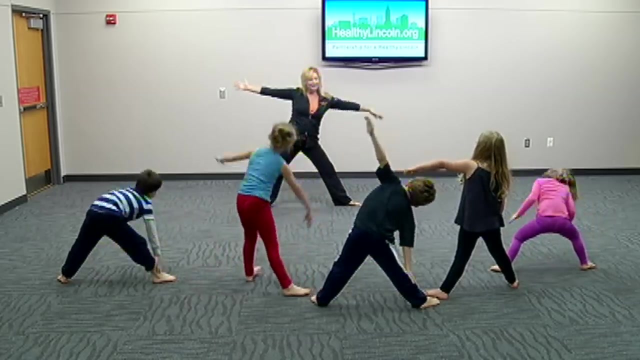 all right, all right. how about triangle? let me make three different triangles with our body. do you step your feet up and then you're gonna slide forward, feet out, and we want one foot to turn out and we're gonna tip that way. whichever way that foots turning, here we are tipping. okay, come back up and turn. 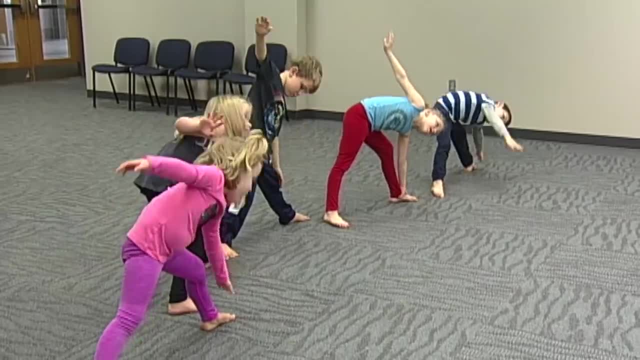 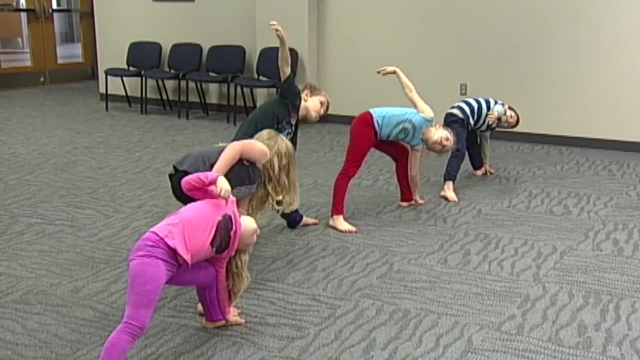 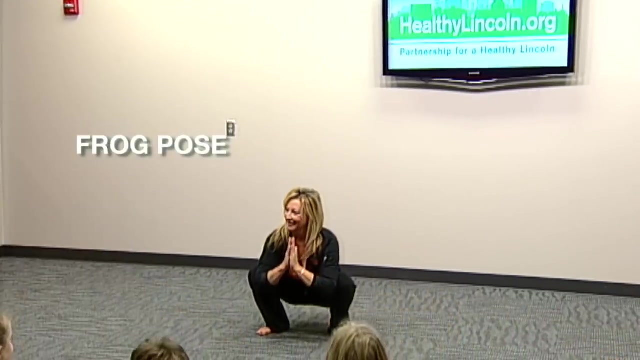 this foot in this one out and go to this side. good, you see all the triangles. yeah, there's even one right here, yep, and from your hand to your feet is another big one. come back up. good, okay, let's come down into frog pose. all right, so we're. 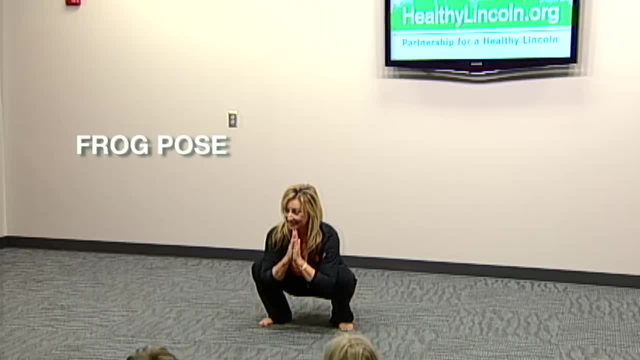 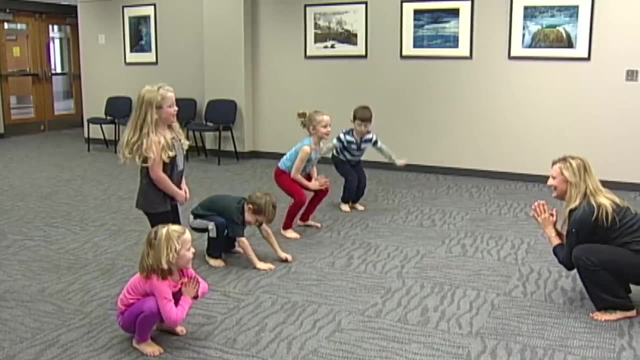 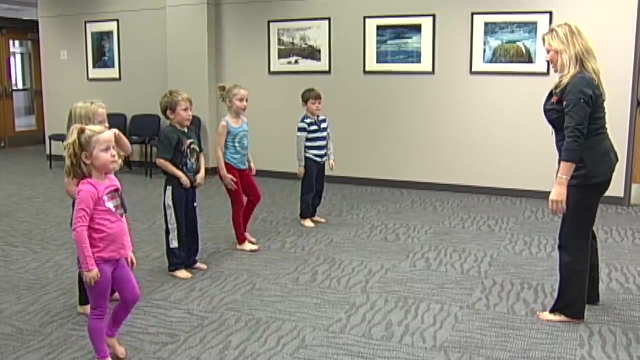 gonna hop and rib it three times in our frog pose, as high as we can. so take a deep breath in you, ready, here we go, all right. so let's go ahead and bring it back up to standing. all right, so working with our breath again, making sure we're. 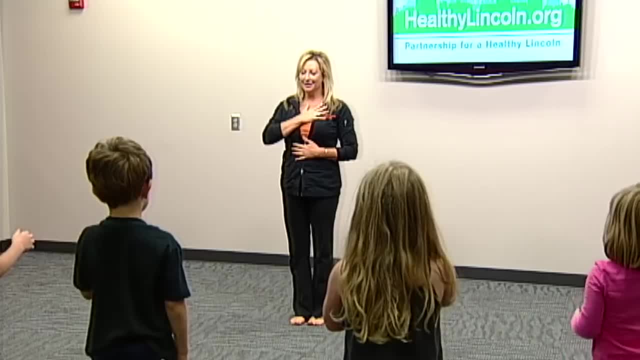 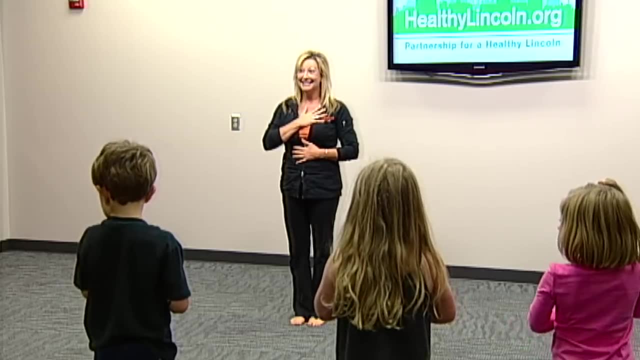 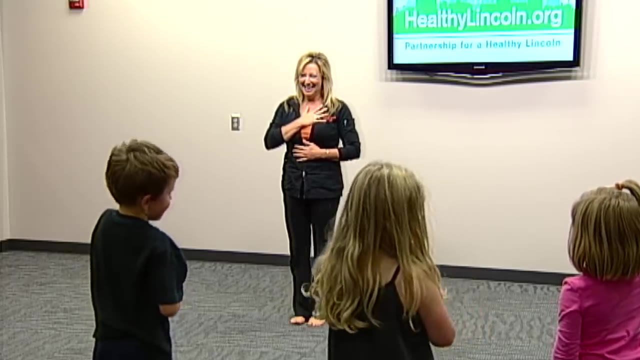 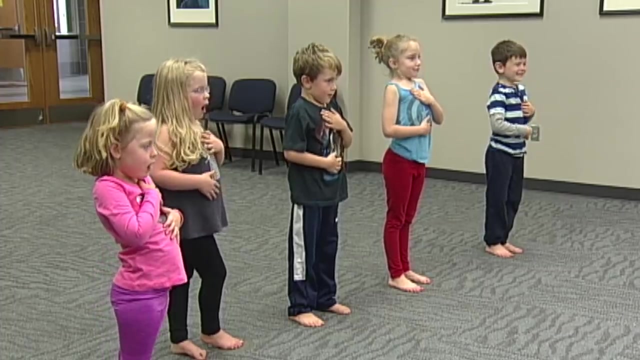 taking nice deep breaths. put one hand on your heart, one hand on your stomach, good. and when you breathe in, do you feel your tummy moving? do you feel your heart beating? that's good. good. and so, feeling your tummy move in and out when we breathe, okay, good. so let's. 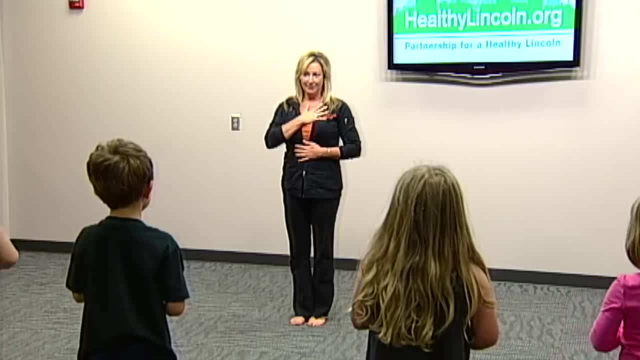 go ahead and work with another balancing pose, so it's called eagle. so let's go ahead and work with another balancing pose, so it's called eagle. so so let's go ahead and work with another balancing pose, so it's called eagle. so sometimes we balance really well. so sometimes we balance really well. so sometimes we balance really well. sometimes we don't and we need to be. sometimes we don't and we need to be. sometimes we don't and we need to be patient and kind with ourselves. so our patient and kind with ourselves, so our 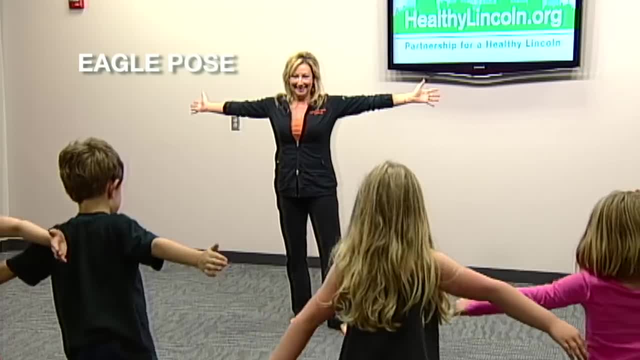 patient and kind with ourselves. so our eagle wings come out, we're gonna take eagle wings come out, we're gonna take eagle wings come out. we're gonna take one foot out and we're gonna wrap this one foot out. and we're gonna wrap this one foot out and we're gonna wrap this foot around and now wrap opposites. so 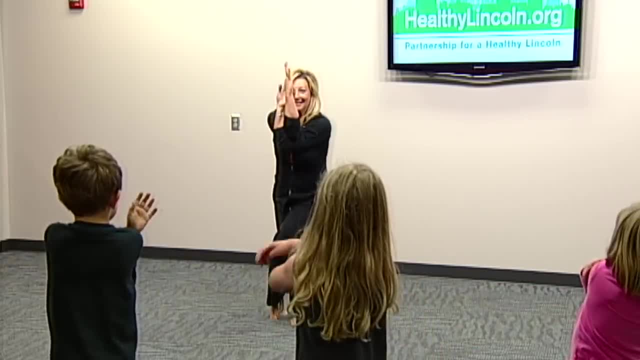 foot around and now wrap opposites. so foot around and now wrap opposites. so this legs on top, this arm comes on top. this legs on top, this arm comes on top, this legs on top, this arm comes on top. good, and we're sitting on our eagle. 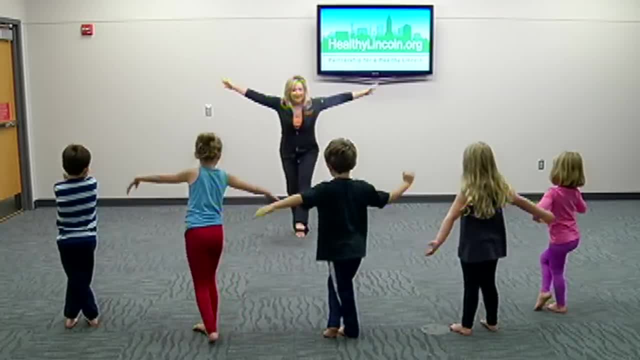 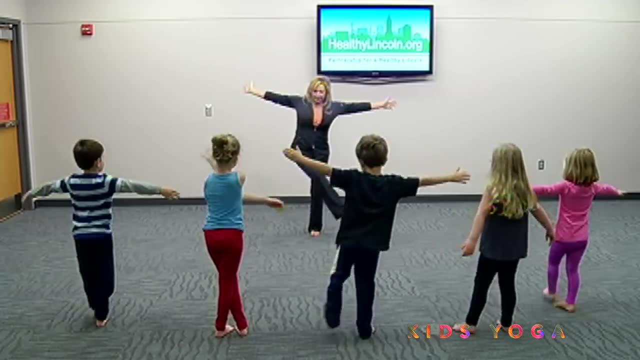 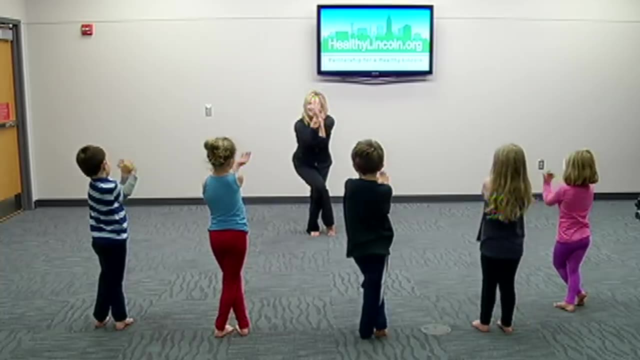 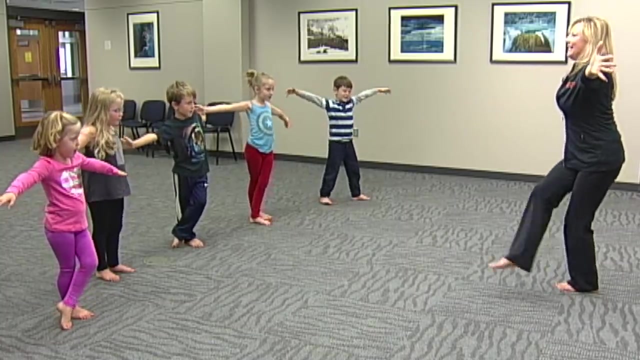 again, here we go, ready, under your wings and flying and step your feet together. let's try the other side. all right, so wings come out, wrap this leg around so we're back into our chair. right, we're coming down and now wrapping the arm opposite arm on top. breathe and now take your wings out and good, let's reach up. 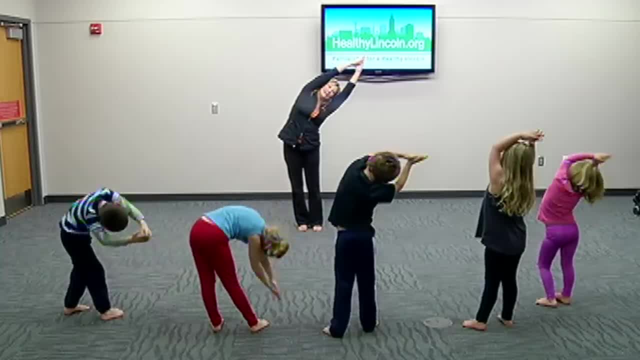 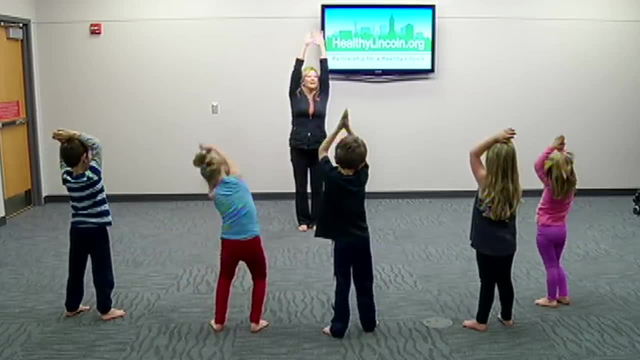 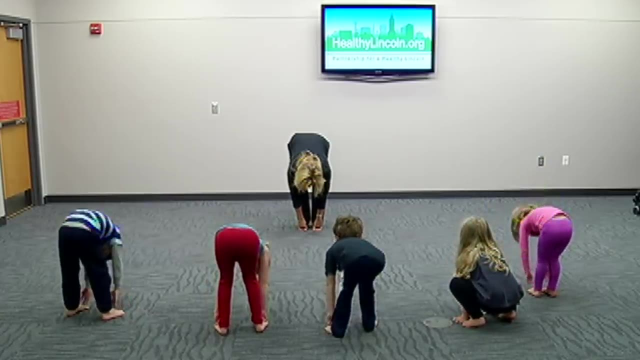 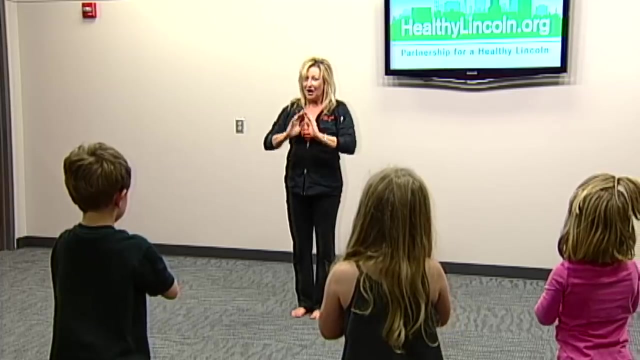 and lean to one side. stretch the side of your body, reach back up and lean to the other side. and back up and fold all the way down. take a bow for all of your good poses, your yoga practice. nice job hands come to our heart. alright, let's. 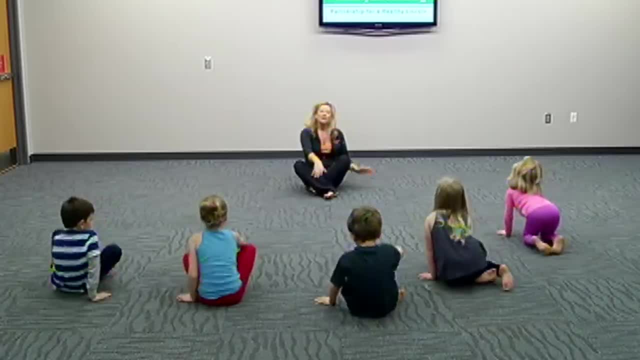 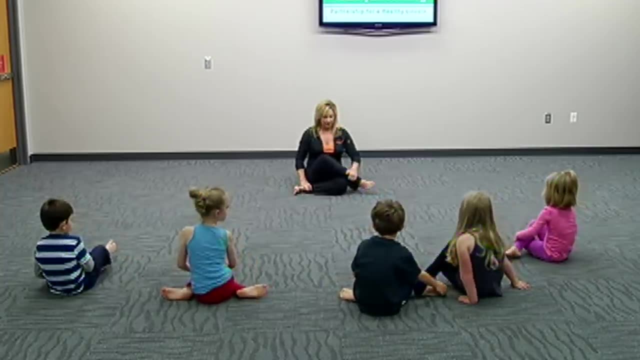 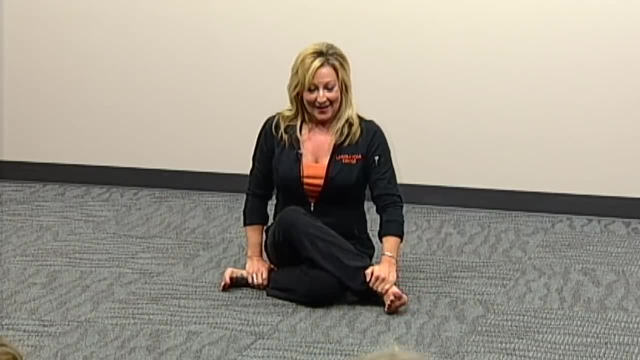 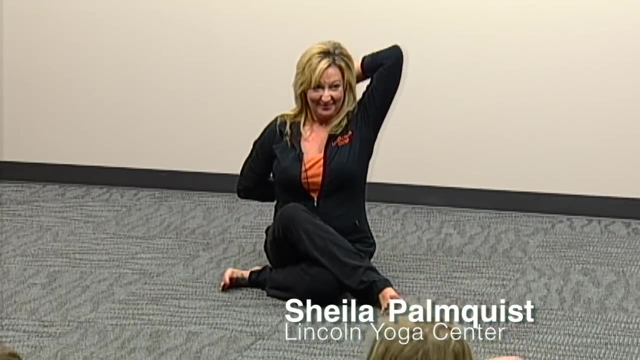 if that doesn't work for you, All right. So take one arm up and fold back And reach back. Some of you may be able to touch your fingers. I can't. I have short arms. Good, OK, lean forward a little bit. 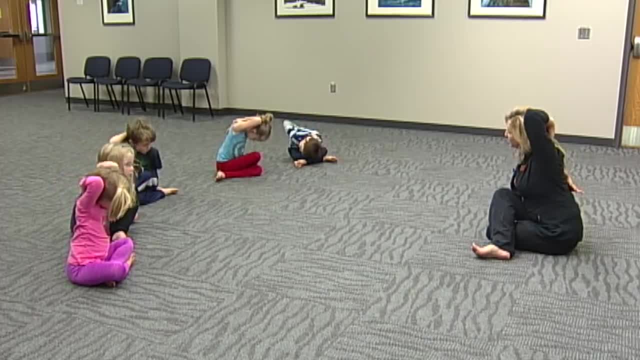 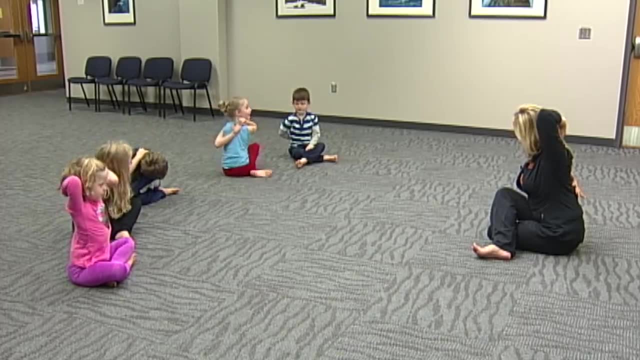 Do you feel a stretch when you start to lean forward? Warm, Yeah, we want to move slowly and gently So that when we feel a stretch, we stop My arm muscles and my leg muscles. You got it. There's a lot happening. 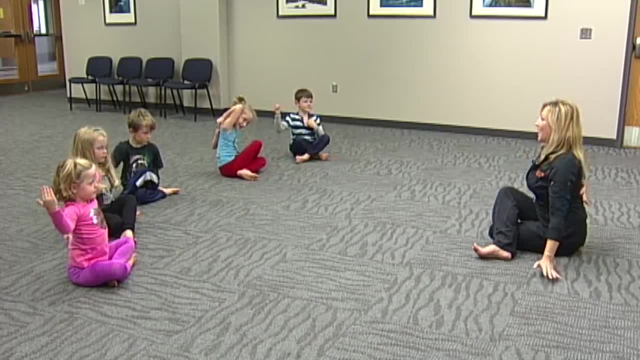 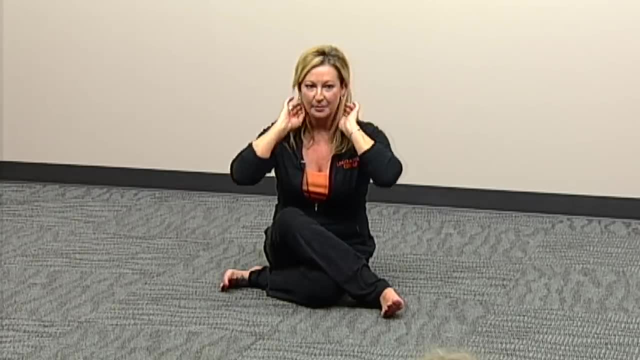 Good job, All right, come back up. Take your arms down, All right. so if you keep your feet down on the floor and you stay low when I spin around, my other leg should come on top. It's called the spin up. 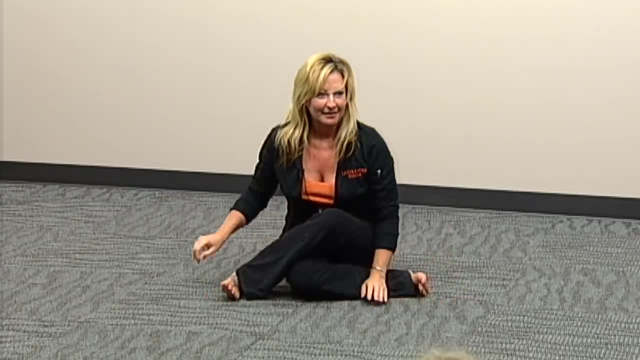 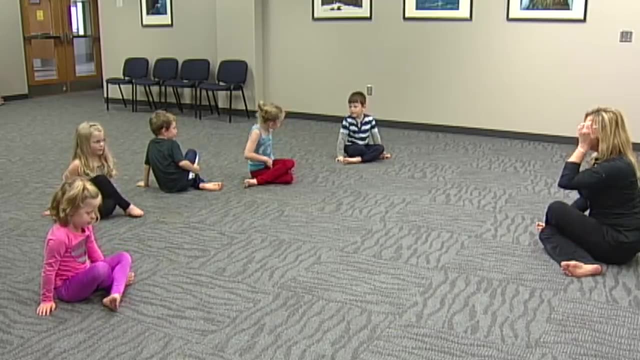 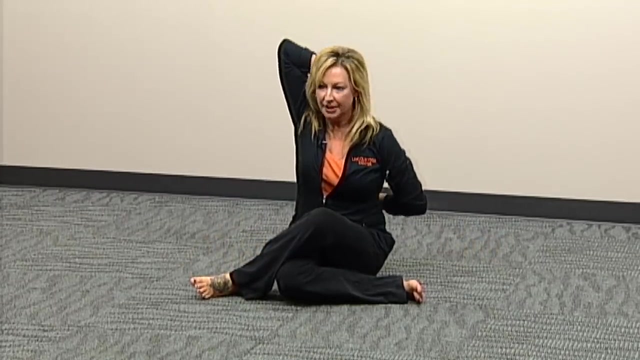 You ready for this? Voila Cool, They're speechless. Good, Nice. So it's fun to experiment and see how does my body move And what would that shape look like in my body? So bringing our arms up again, reaching back, leaning forward. 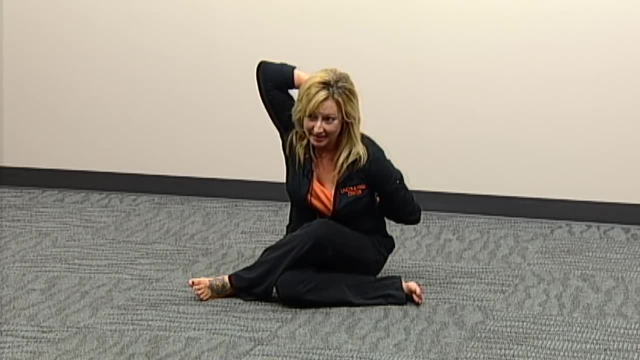 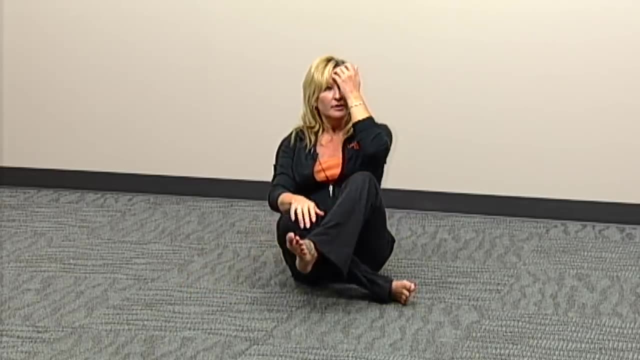 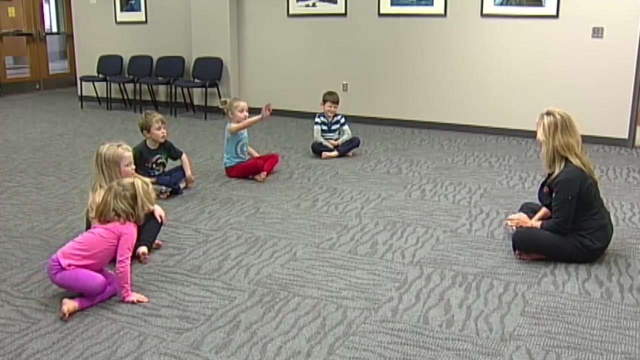 So we're going to do one side and then the other, because yoga is all about balance. Good, And come back up. So we find balance in our bodies, right. So what other areas can we try to find balance On our hands? 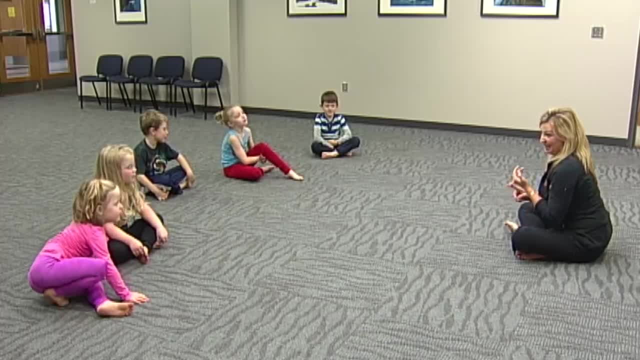 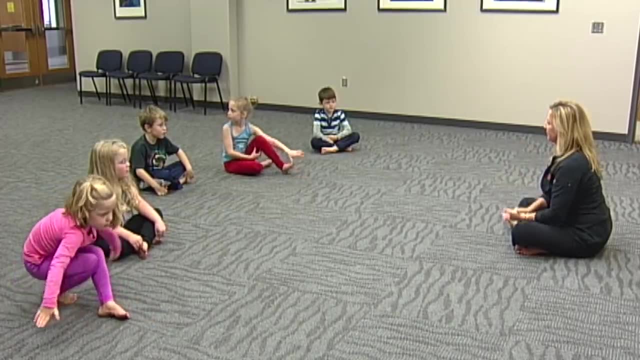 Yeah, we can balance on our hands, Yep, And also what we eat right And the activities we do. So sometimes when we feel like, ah, I'm doing too much, I need to rest. So all of those different places in our lives. 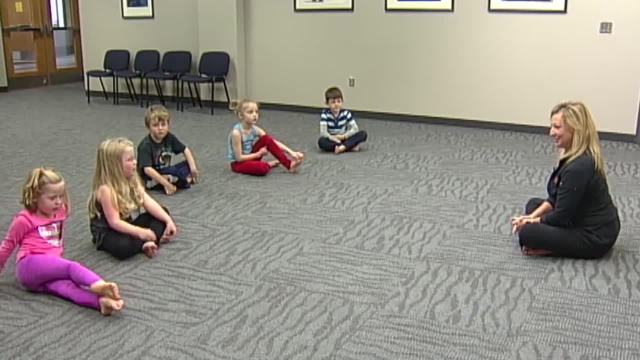 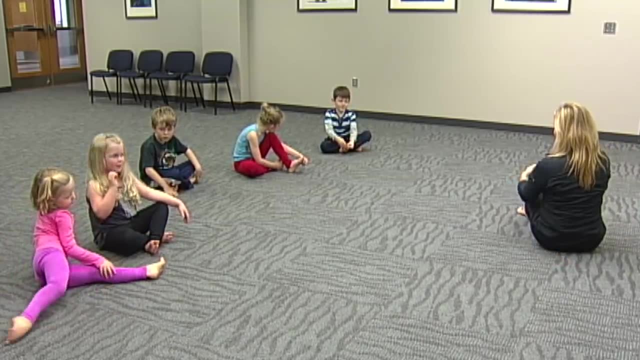 we can try to find balance right. I can balance on my feet. Good job Like Good Like in tree pose. Like I can balance on my feet, Let's go ahead and do bridge. So we're going to roll down. 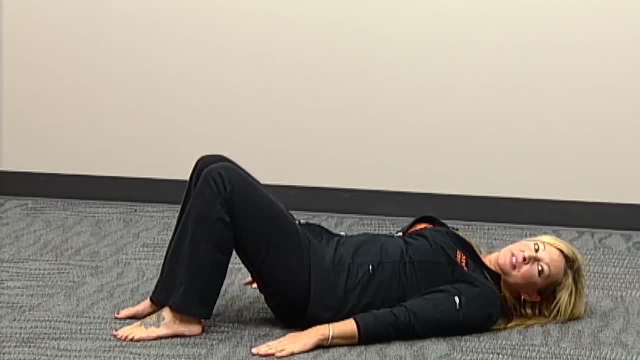 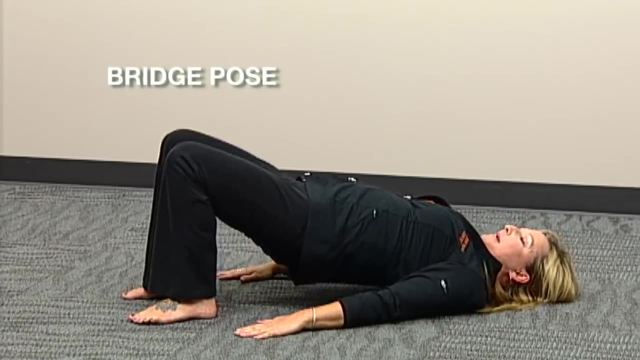 Bridge pose that you do in gymnastics is different than bridge pose in yoga, So we don't want to rest our weight on our neck. That's kind of dangerous. So our hands stay down, So watch me first. And we're going to lift up like this. 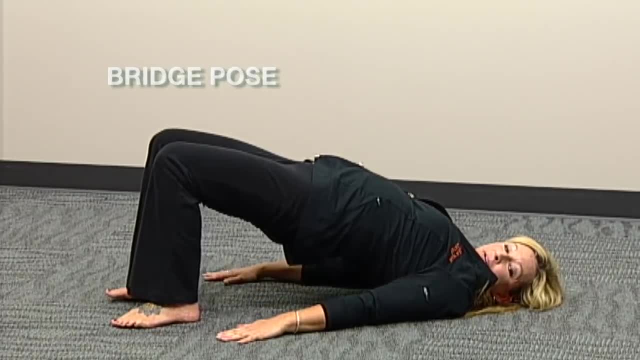 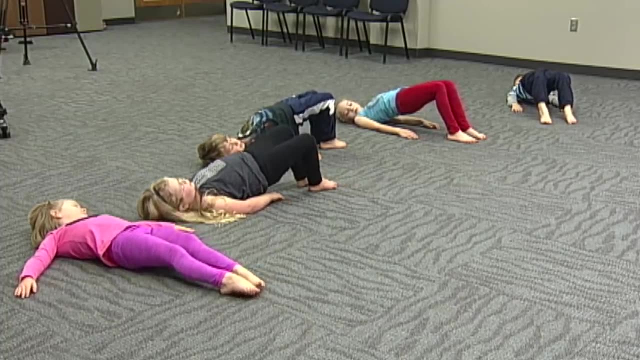 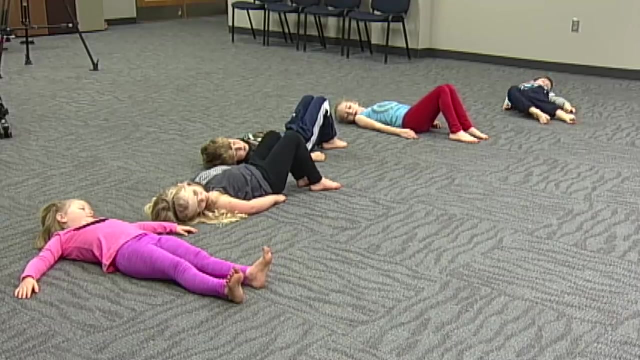 So you're lifting your bridge like you could drive car underneath your back. Good, Come up and then come back down. Good, One more time. Lift up in your bridge pose and lower your bridge back down. Good, OK. Next one is happy baby. 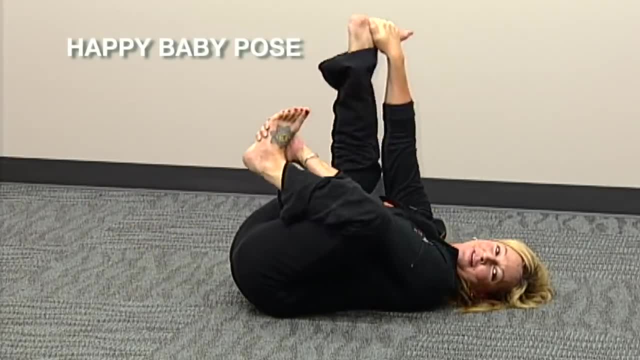 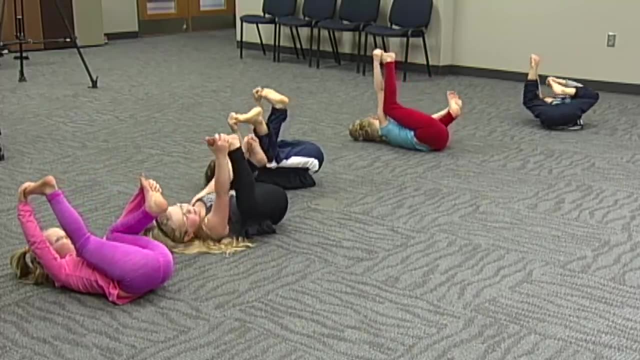 So we grab our feet and stretch back and forth, Back and forth. Happy baby. So again being playful, right, Yeah, Yeah, Yeah, Yeah, Yeah, Yeah, Yeah, It's a good stretch too, All right. 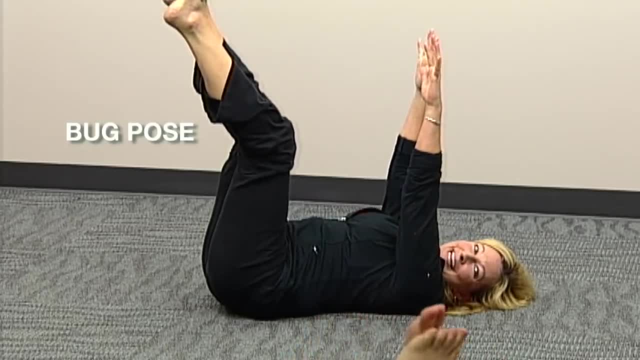 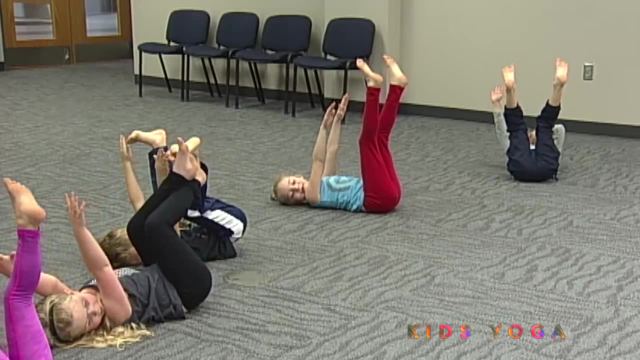 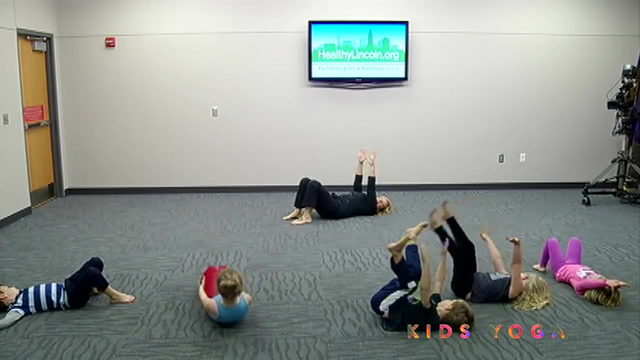 Now our arms and legs are up towards the ceiling. This is called bug pose, Like a bug stuck on its back. Good, Or like that. Yeah, Yeah, Or that. Good job, All right. So bring your feet down And you're going to roll down. 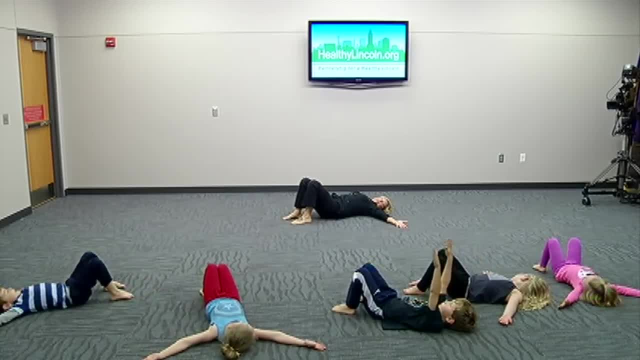 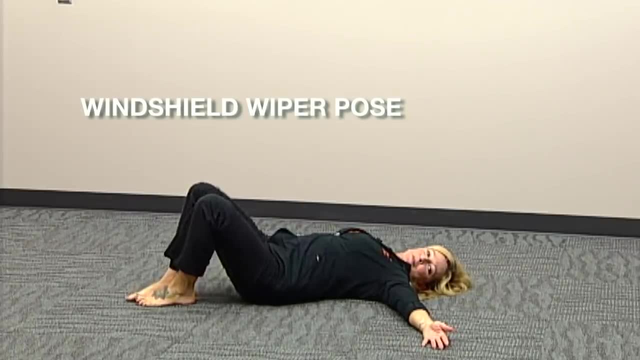 And your arms out nice and wide. Good, And now windshield wipers. Let your knees go to one side And bring them back up, And to the other side. Windshield wipers, Back and forth, Back and forth, And this should feel good on your back. 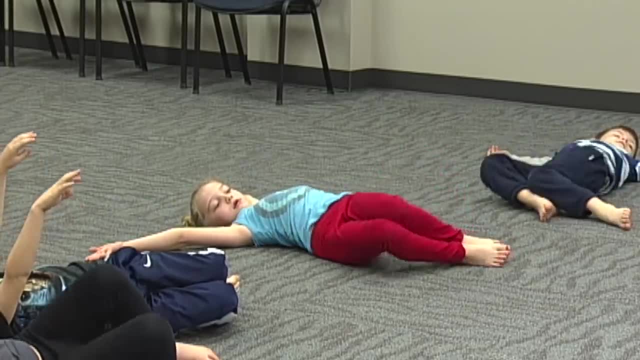 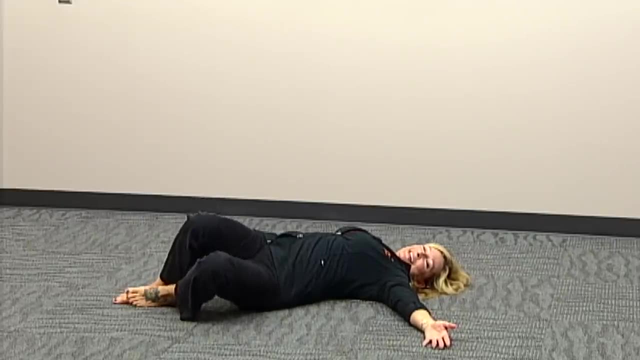 Right. Does it feel good? If it doesn't feel good, then we want to do it differently or not do it at all. if it hurts, It feels weird, Good, All right, So we're going to roll it up from here. 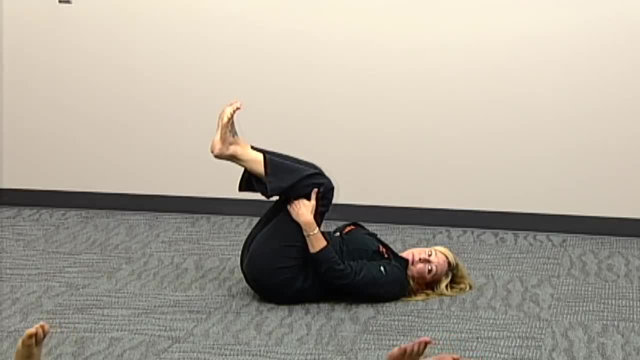 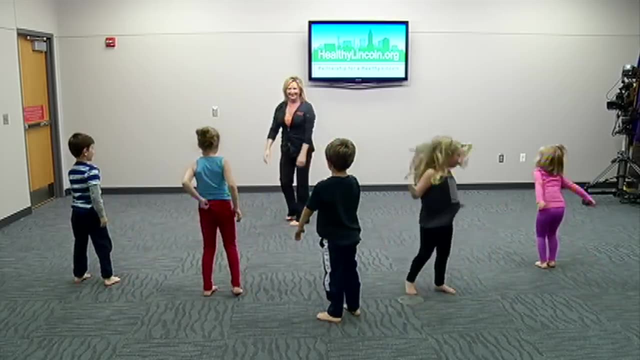 So let's see if we can come all the way up to standing. You think you can get enough momentum and come up to standing? Yeah, All right. So here we go, Roll it up. Good, We made it All right. 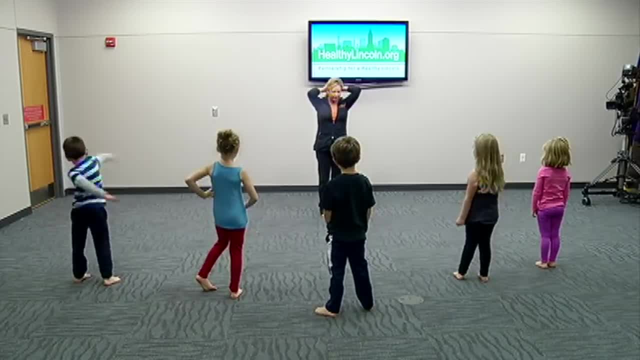 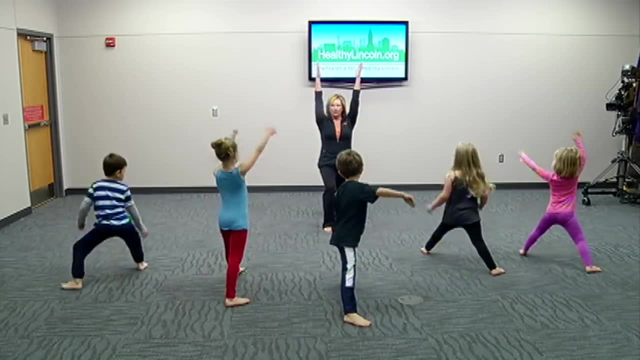 So let's do a couple more stretches standing And then we'll move down to the floor and do our relaxation. So bring one leg forward, One leg back, Bend your knee and bring your arms up. Warrior one Good, Super strong, powerful warriors, right. 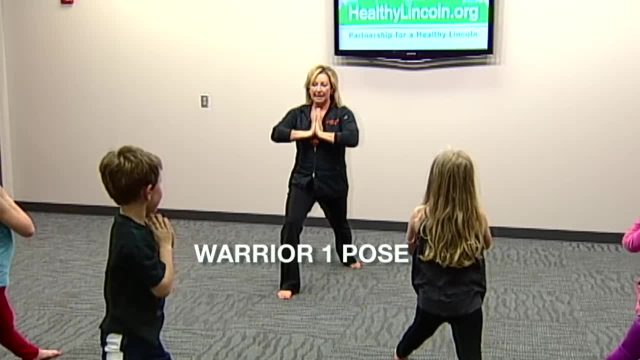 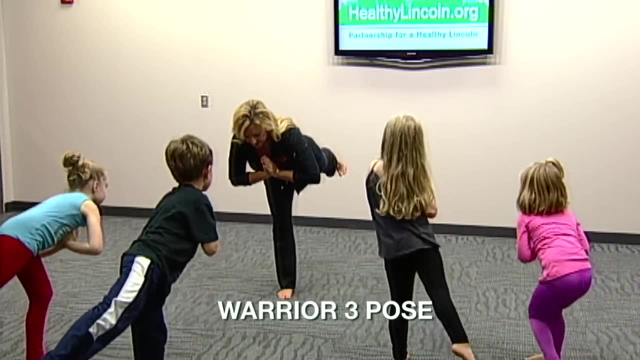 And now Hands come down this way And we're going to take this into warrior three. So here we go, Lift your back leg. We did this one with. I am balanced right, But we had our hands different. Good job. 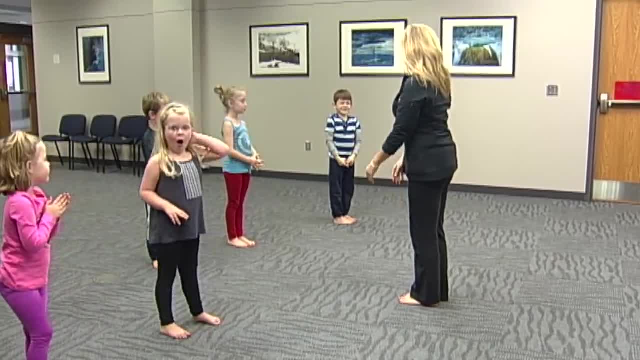 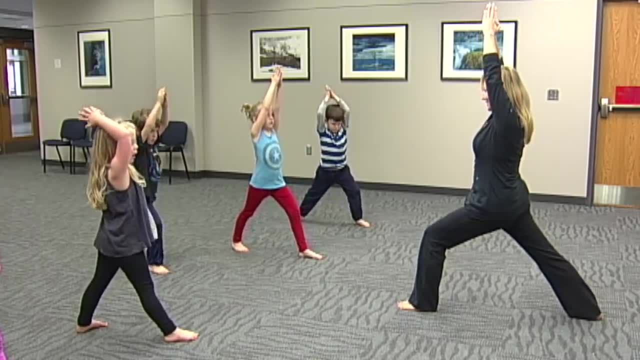 Step your feet together. I think it's warrior three. Yep, Let's do the other side. Step back, Bend your front knee, Take your arms up over your head in warrior one. Good, This is easy. Good Hands come to heart center. 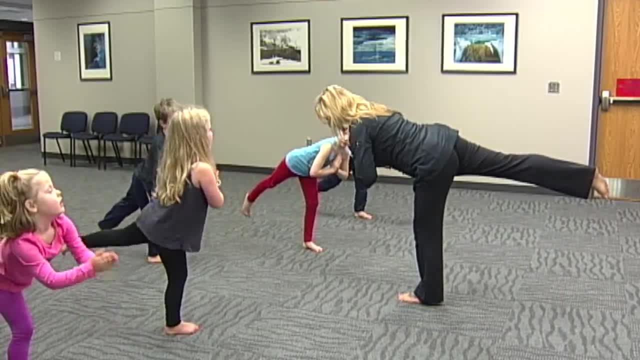 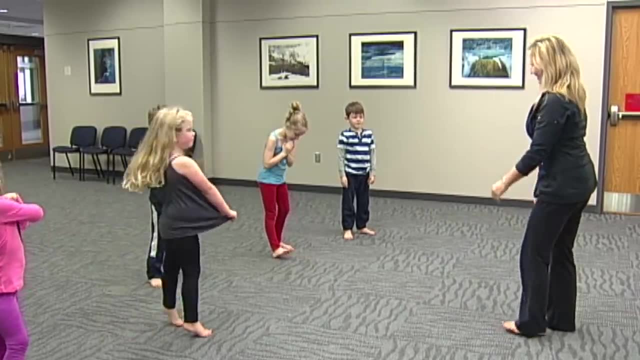 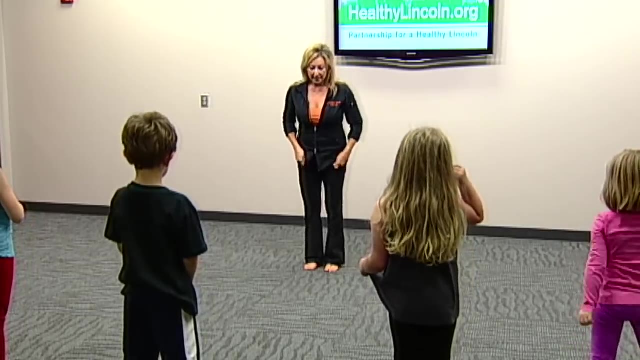 And lift your back leg, Good job. Step your feet down, Nice, All right. Yeah, All right. We need our eyes and our muscles and our ears, our inner ears, to help us balance, All right, So let's do one more breathing practice. 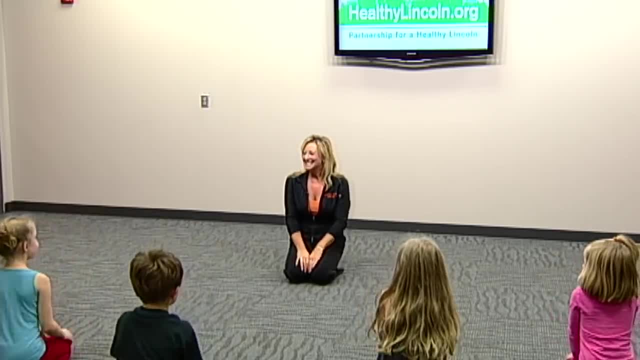 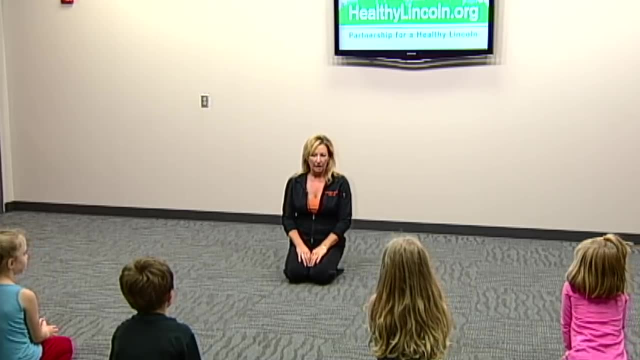 So, coming down here, we're going to do buzzing bee- Yes, Buzzing bee breath Yep, And so it's a little bit deeper than a hum. So have you ever done this? Ah, Yeah, Ah, Ah, We've all done that. 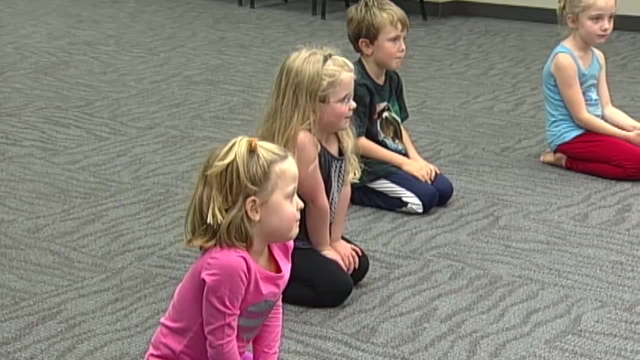 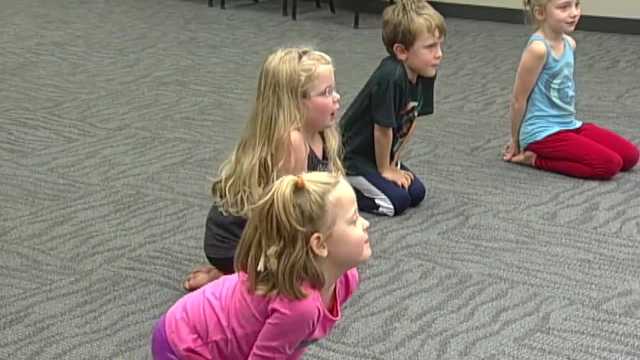 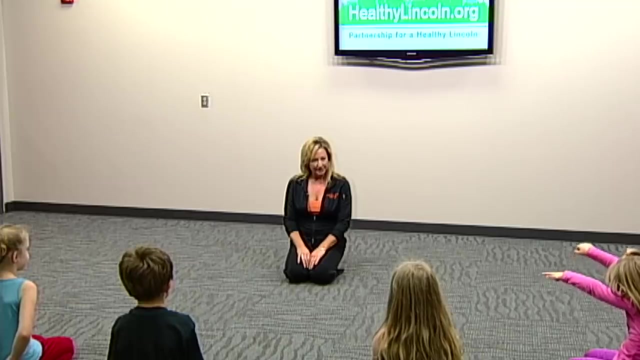 So try to do it with your mouth closed. Mm, It kind of tickles your nose right, Mm. Good, All right. So with buzzing bee we're going to close our eyes and our ears. So imagine you're a bumblebee flying over a field of flowers. 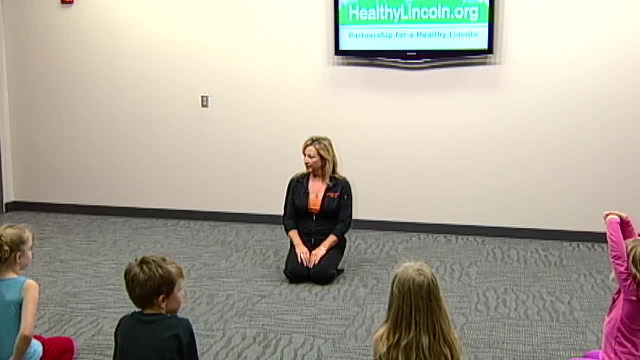 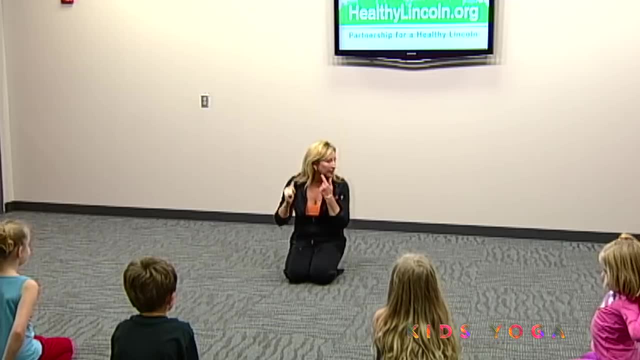 We're going to do it one time. We're going to buzz out as long as we can when we breathe out and then wait for everyone to finish, So we actually use our thumbs to press against this part of our ear, so we don't stick our thumbs in our ear. 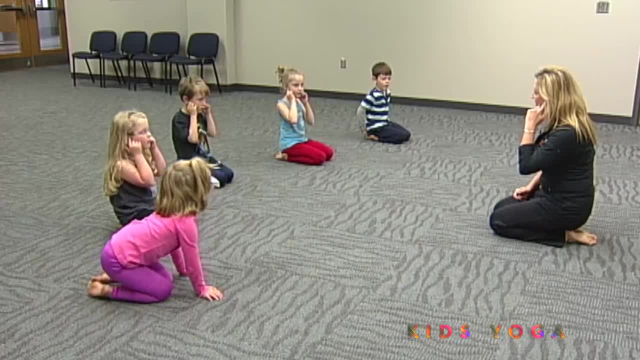 But you see this kind of hard piece right here. Go ahead and touch it. That's cartilage of your ear. You're going to press against that and then just gently lay your fingers over your eyes. We don't want to push too hard. 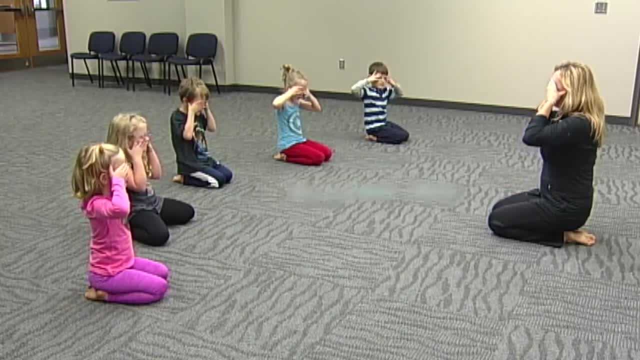 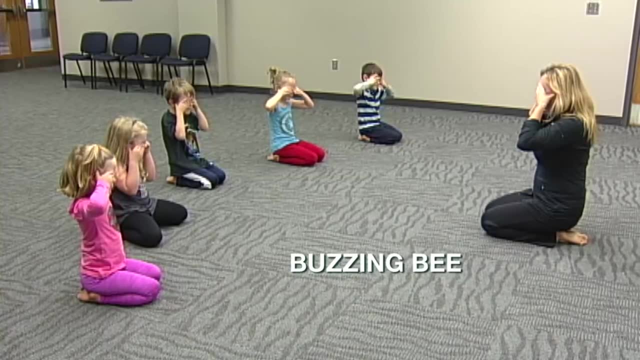 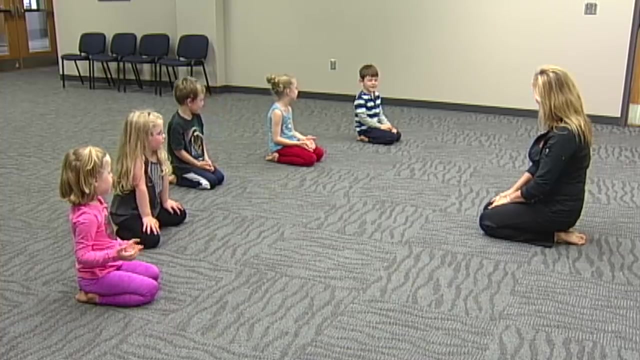 And then we're going to do one buzzing bee. OK, you ready, Here we go. It sounds like a bee And our hands come down. Good, It really does sound like a bee. It does, I know. Look at how that just calmed us all down right. 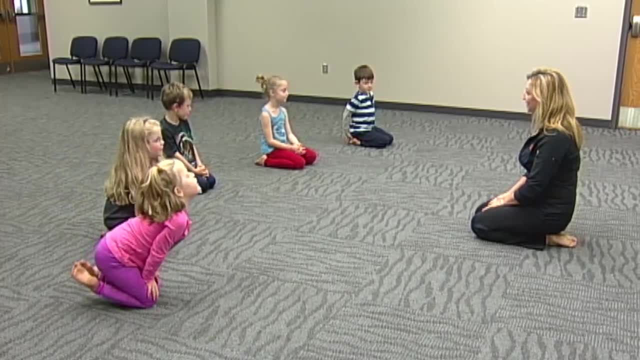 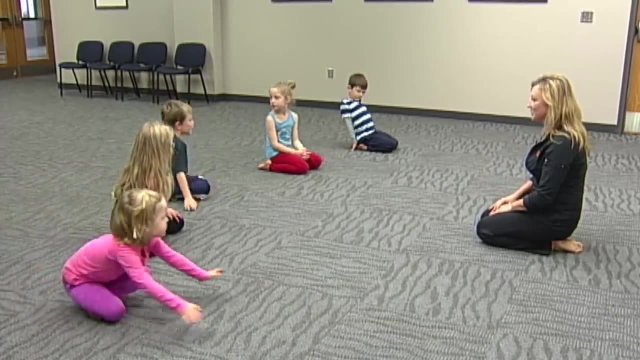 It's calming It is. yeah, We can use our breath to wake us up, to calm us down, to cool us- all kinds of good things. So let's go ahead and come onto our bellies for a moment in crocodile. 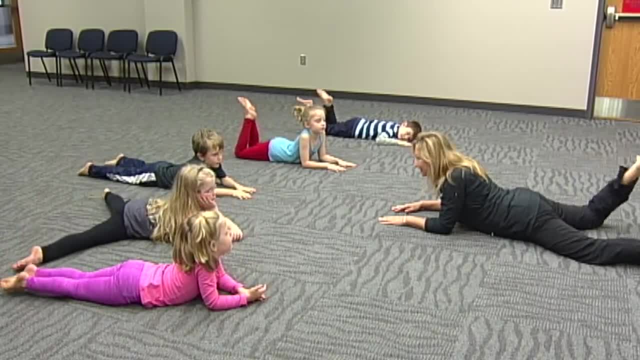 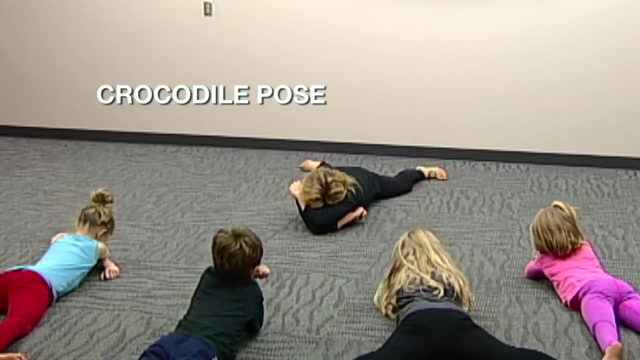 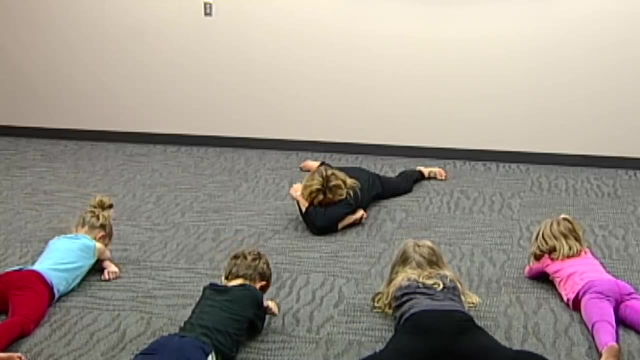 So crocodiles' feet and knees go out like this right. And here's our crocodile mouth: Chomp, chomp. So bring your head down And breathe and relax here like a quiet crocodile. Good, Start to lift your head like you're looking around. 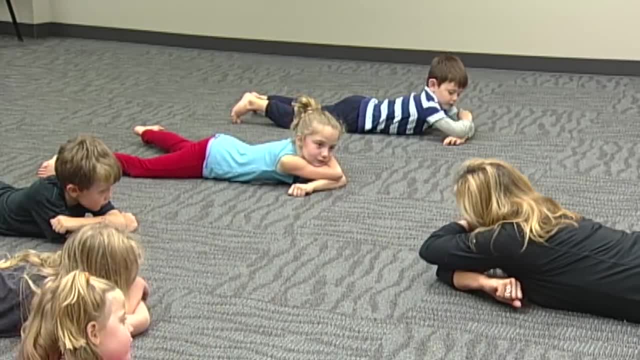 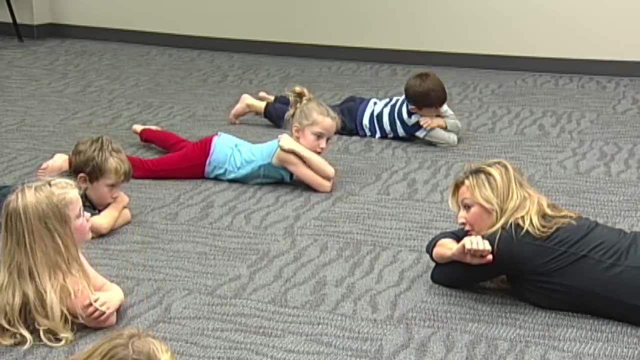 checking things out, right. All right, We're going to take one big chomp, Ready Chomp Chomp, And now switch Other jaw on top. All right, So move your feet a little bit. So crocodiles have that big, strong tail too to take off. 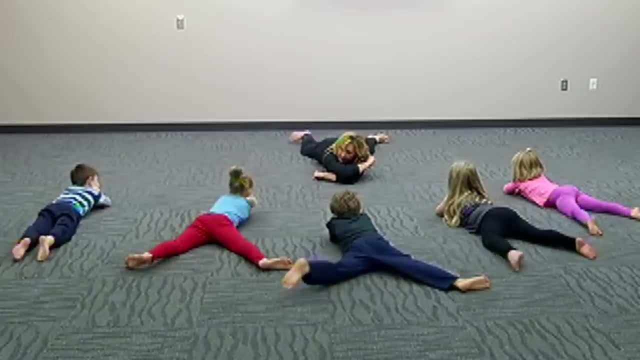 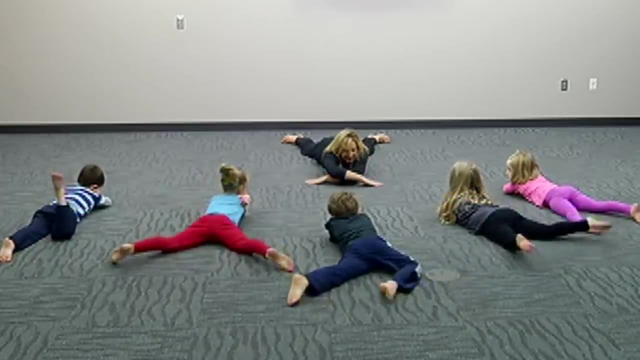 We don't have that, But we have our legs and our feet, So we can wiggle around a little bit. We don't have to be like statues in our yoga poses. We want to move around, All right, So now sweep the arms down. 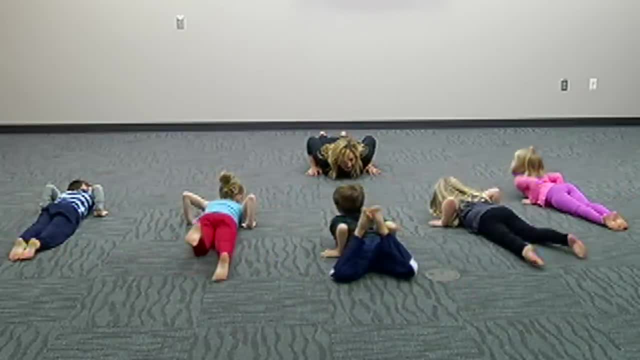 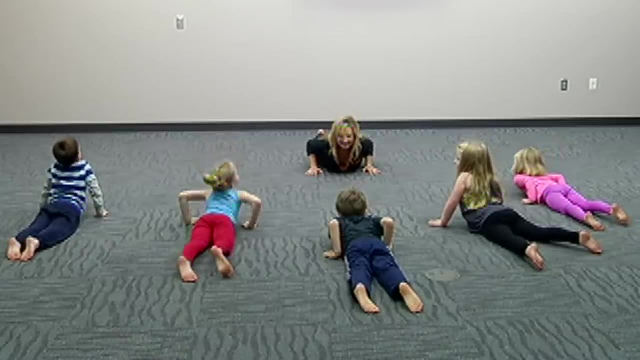 Tops of your legs come back, So your feet come back in And let's go ahead and lift. Here's our cobra again. Yeah, Thank you. Good Breathe out. Ssssssssssssssss, Nice job. 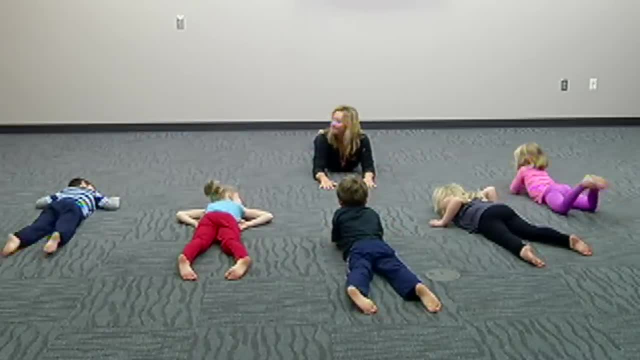 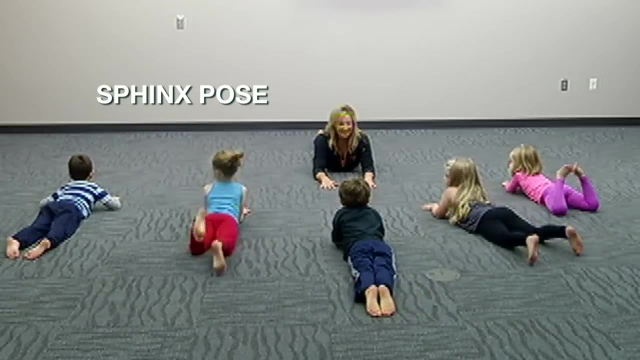 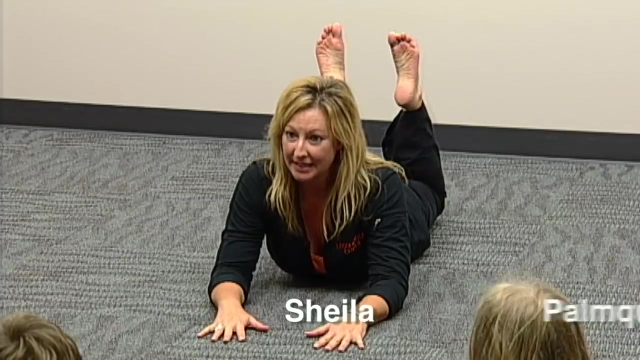 All right. So now take the arms out in front. This is called sphinx pose. All right, Good, We're in sphinx pose. you got it. Yep, Some of you- I've done a lot of yoga with kids- can go here and bring your head back towards your feet. 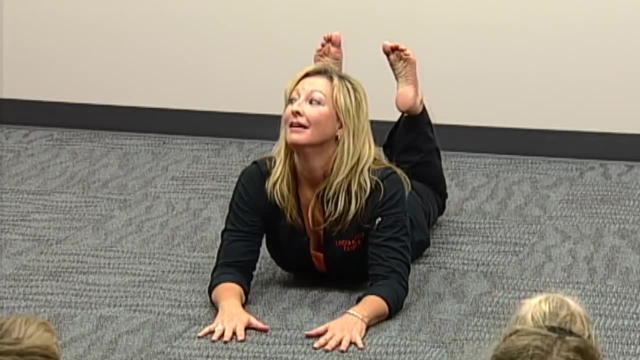 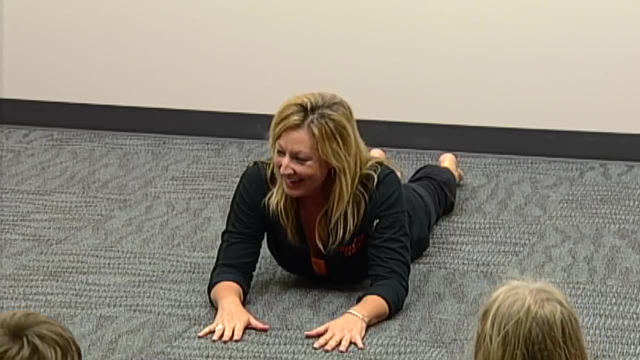 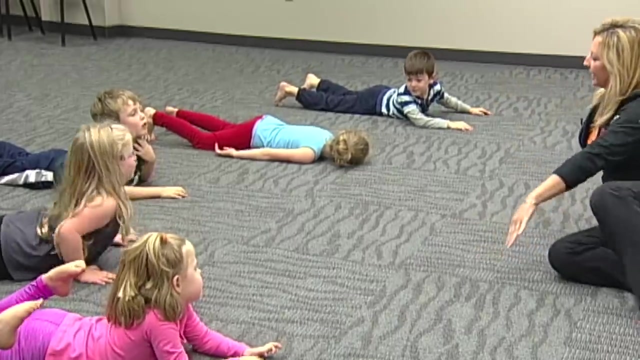 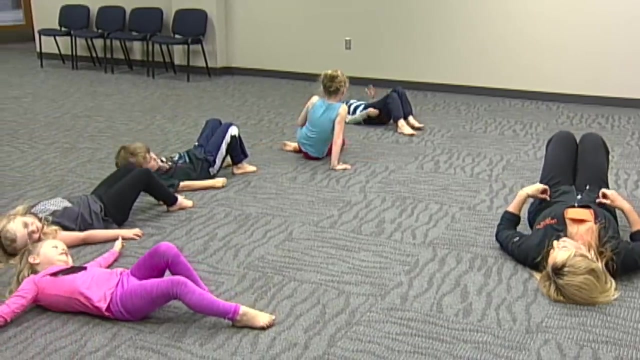 I can't, but you can try if you want. Look at how close you all are. good job, Good, Do you? So we're gonna roll onto our backs now, Okay, so we're gonna come down for our relaxation, So roll down onto your back. Good, we're gonna keep our feet bent for a moment, So our knees bent, so our feet are on the floor and 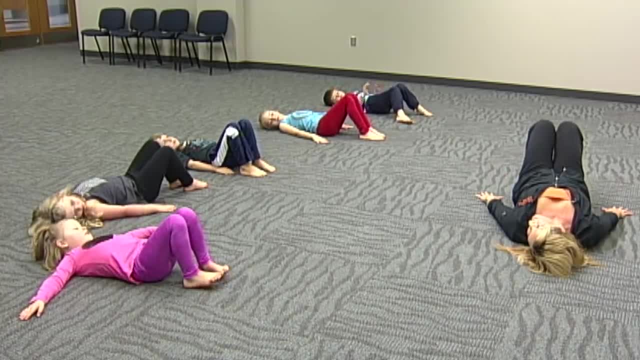 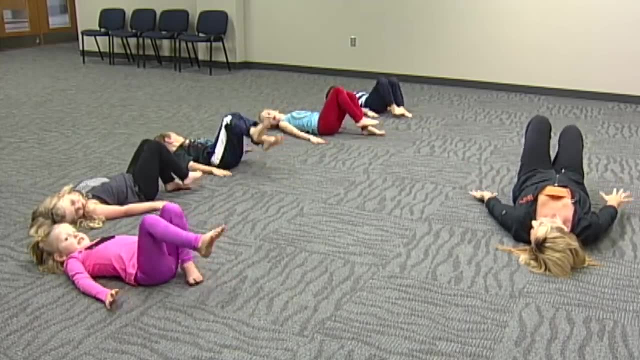 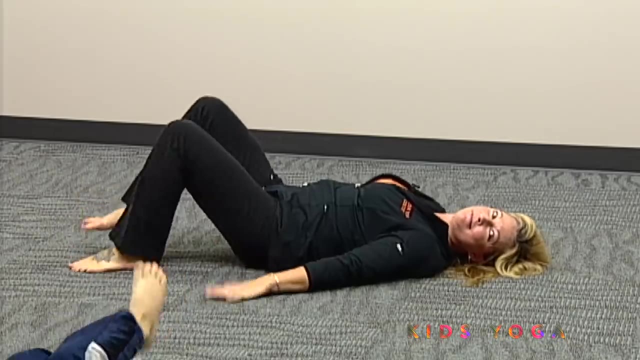 Nope, we already did that. one arms stay down. Okay, And so now we're gonna tap our arms and our feet Ready. here we go, stomp Good and stop and do it one more time, ready Like you're having a tantrum, get out all that frustration and then stop. 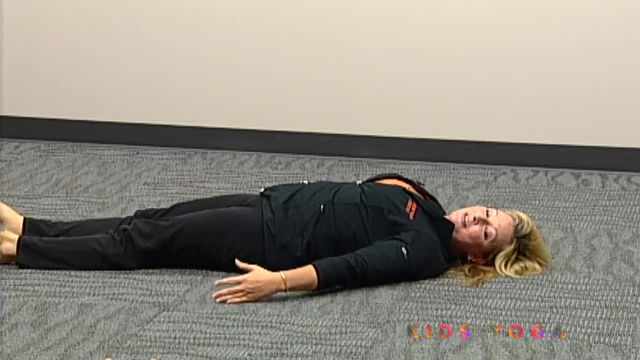 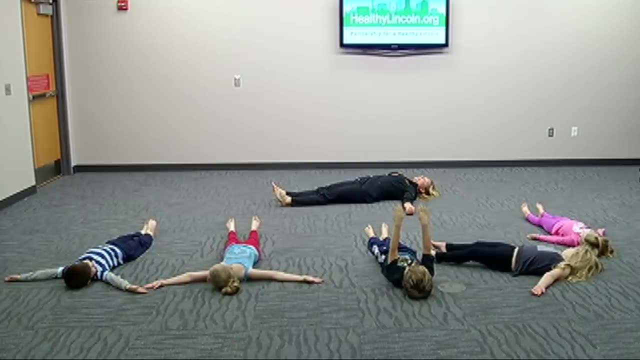 Okay, Now take your legs straight out and Turn your arms up towards the ceiling. Good, Okay, close your eyes and so imagine you're melting into the earth. So this is called earth pose. so your melting down. Notice your breathing. your tummy rises when you breathe in and falls when you breathe out. 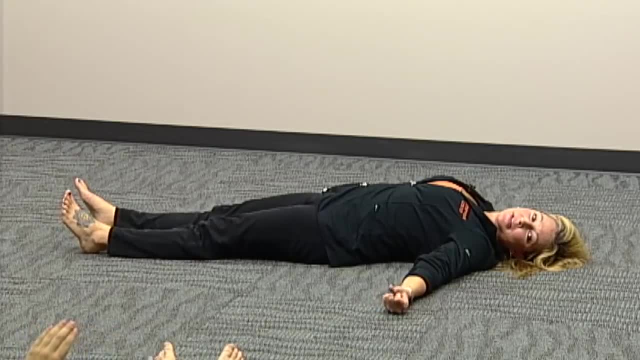 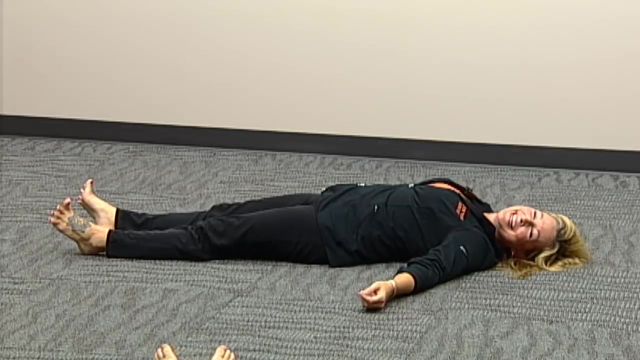 And so now, tighten all the muscles in your body. squeeze your arms, your legs, everything. scrunch up your face and then relax Good one more time. tighten all the muscles, make a fist, scrunch up your toes, Ah, relax, Good. Often this is the best place to have fun. 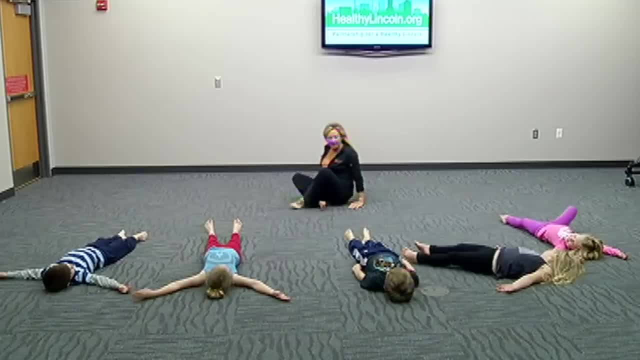 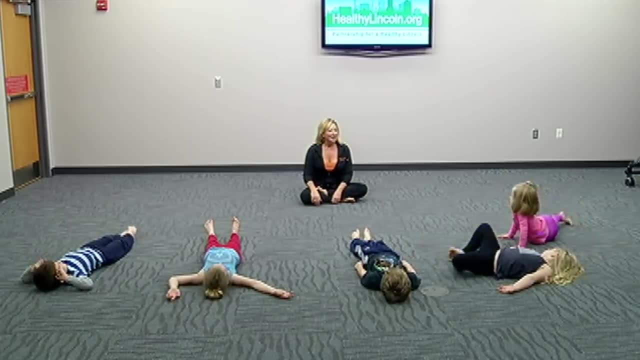 It's when you do some work that keeps your breathing and Settings gets great. Put your hands out and, like this, come up on your white bar, Let the weight of these arms back on your chest Up, bend your arms without finale. So from here I'm gonna sit up, just so you can hear me better. 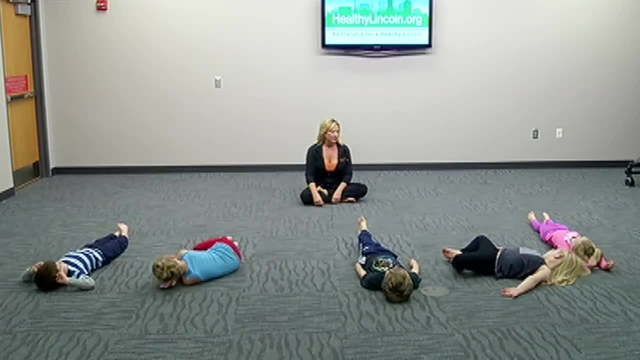 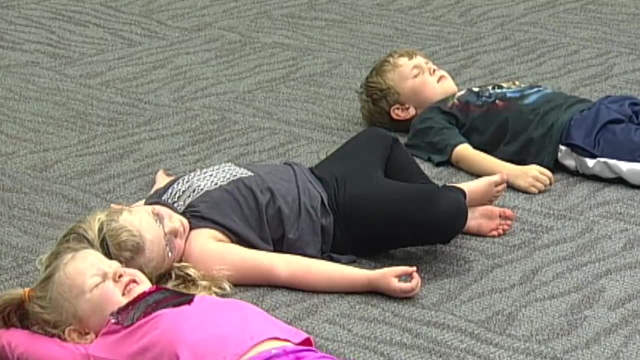 So keep your eyes closed. but now you get to take your own little adventure, like you're riding on a cloud, So closing your eyes and imagine you're floating on a cloud, Good, and then if you could go anywhere you wanted to. so make up your own story here. 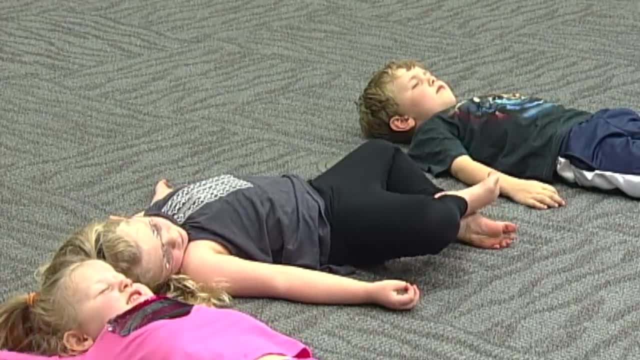 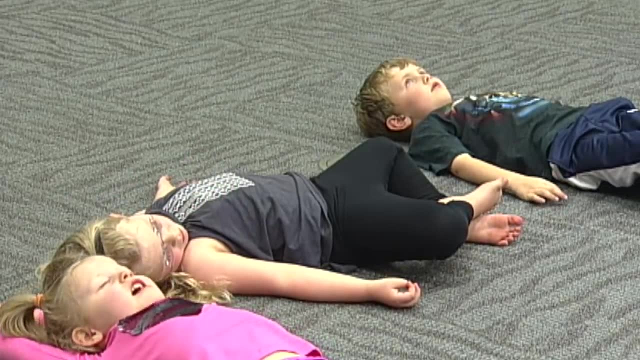 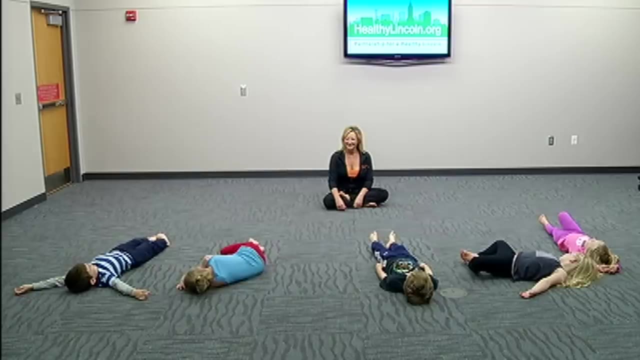 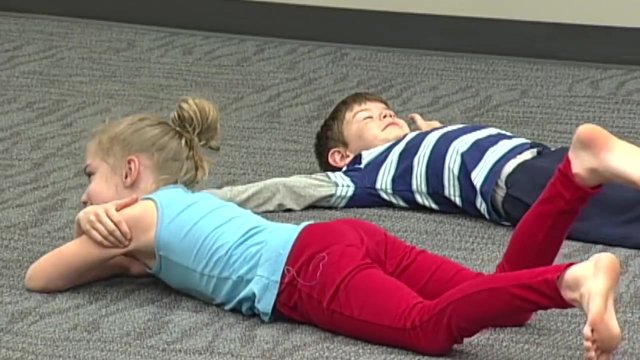 Where would you float to? Would you go over mountains and oceans? Maybe you'd go to the pyramids, to Egypt, Maybe you'd go all the way up into space, any place you imagine Good. and so, after you've had this really cool adventure, you start to make your way. 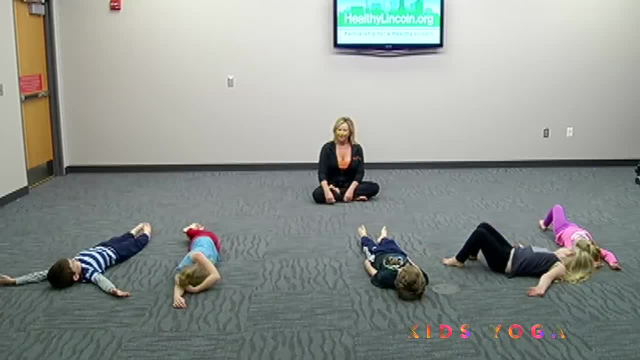 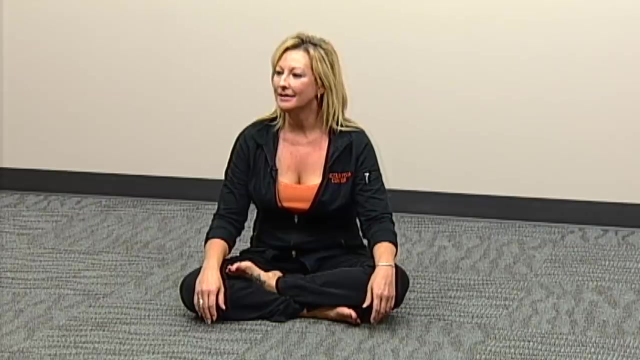 with your cloud back towards Nebraska, floating back over the cornfields, Good, Back over the building, and you start to float down through the ceiling. so you have to take deep breaths out so your cloud can lower down, Little bit lower, little bit lower, and imagining you're rolling off of your cloud and start